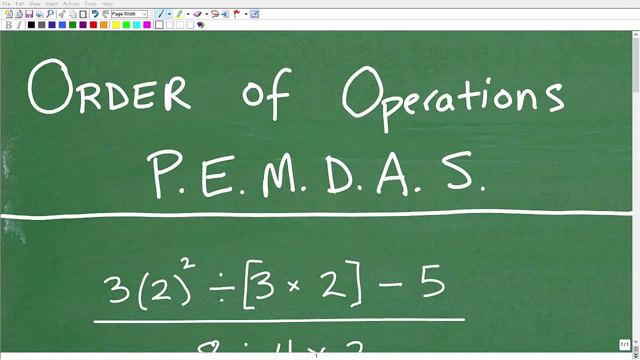 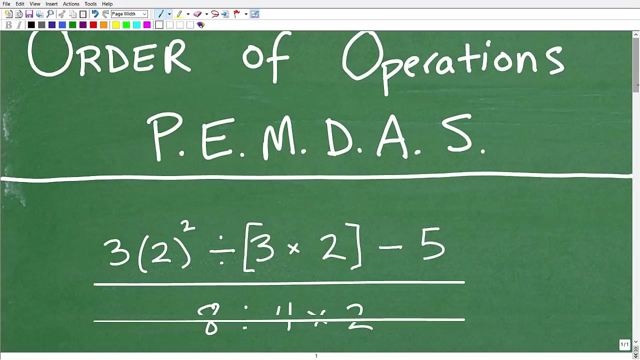 Okay, let's talk about the order of operations, And many of you out there know it by this acronym, PEMDAS or PEMDAS. I'll get into that in a second, But I'd have to say that the order of operations is an area where many, many students think they understand it better than they actually do. So we're going to take a look at a practice problem, And here it is. We're going to go through and simplify this using the order of operations. 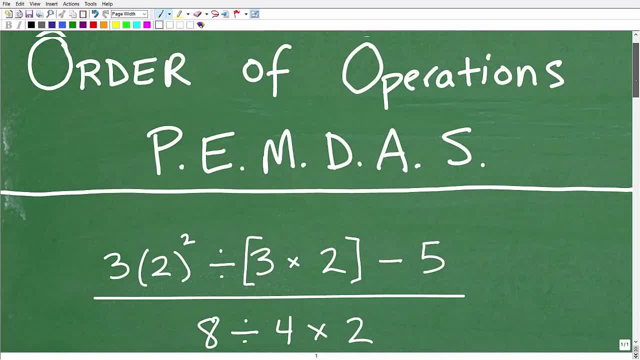 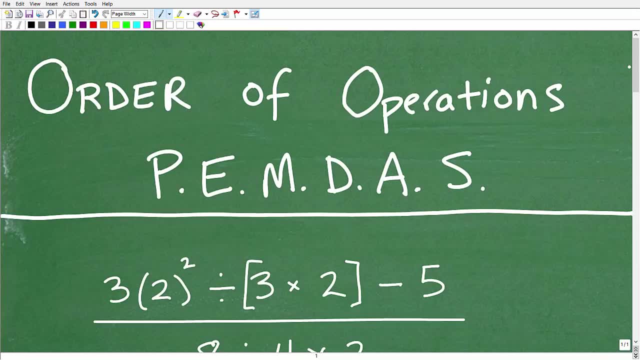 Just to kind of review some of the things that you really need to understand. I would say again that this is an area where it just trips up so many math students. So if you can really strengthen your understanding of the order of operations- just do a quick review and make sure you truly understand it- then that's going to help you out in math for sure. 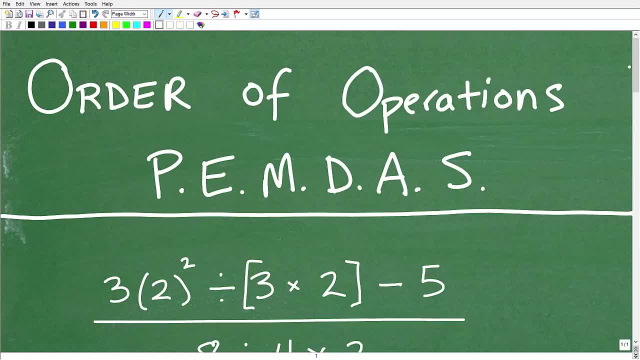 So before we get started, let me go ahead and introduce myself. My name is John. I'm the founder of Tablet Class Math. I'm also a middle and high school math teacher And over the last several years I've constructed many online math classes to include several middle and again high school math classes. 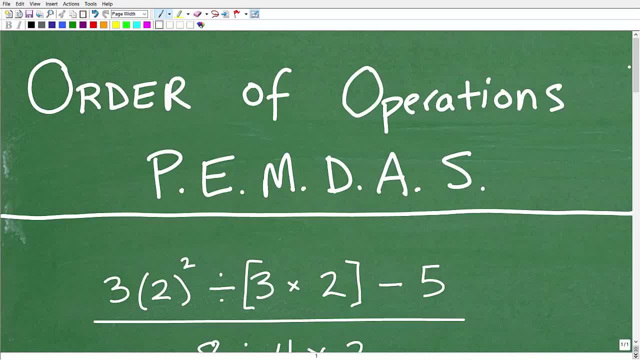 So the order of operations is typically taught at the middle school level. It's really kind of honed in there. So if you're in that range- middle school range- you might want to check out my pre-algebra class, for example. 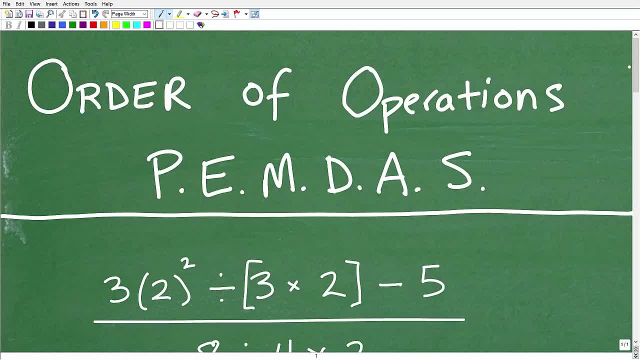 But nevertheless, I'm going to leave a link in the description of this video to my math learning program And you could see you know if there's a course there that might be right for you. Also, I'm going to invite you to become a subscriber to my YouTube channel. 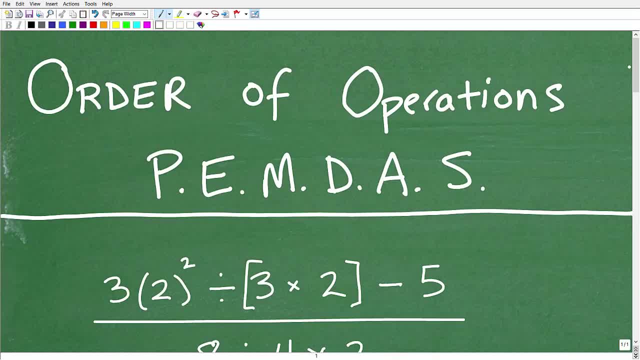 I already have hundreds of videos on my YouTube channel posting stuff all the time. I love to teach math, So if you like my teaching style, I probably already have a lot of stuff there that can help you out through your course. And again, if you like this video, please consider giving a big thumbs up. 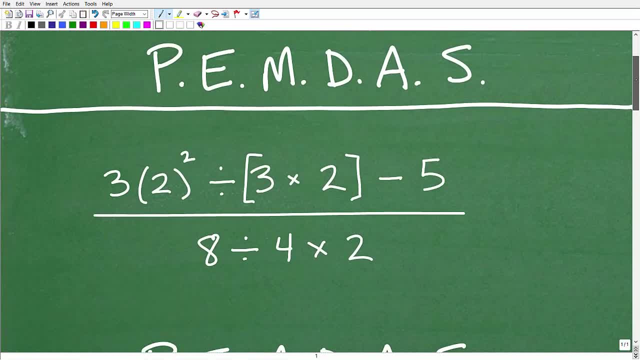 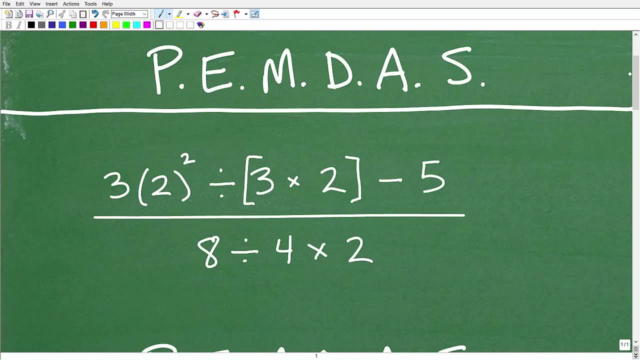 All right, So let's get into the problem. All right, So here is the problem. OK, And I'm not going to recite it, but here it is, And I wouldn't. I suggest that all of you out there, you know, pause the video and just go ahead and knock this problem out. 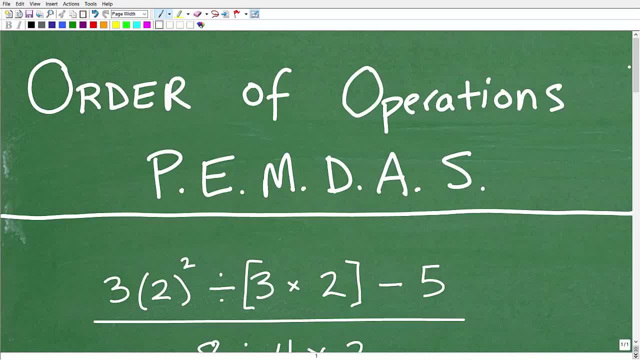 So the order of operations is typically taught at the middle school level. It's really kind of honed in there. So if you're in that range- middle school range- you might want to check out my pre-algebra class, for example. 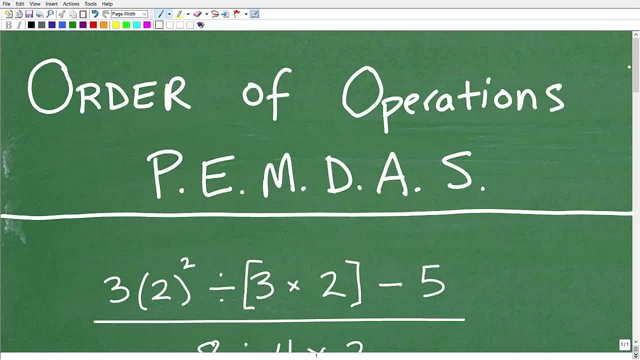 But nevertheless, I'm going to leave a link in the description of this video to my math learning program And you could see you know if there's a course there that might be right for you. Also, I'm going to invite you to become a subscriber to my YouTube channel. 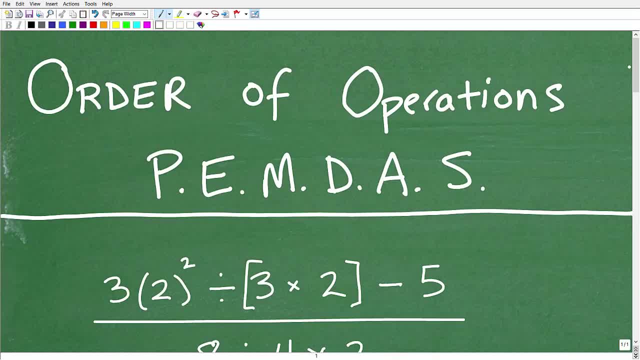 I already have hundreds of videos on my YouTube channel posting stuff all the time. I love to teach math, So if you like my teaching style, I probably already have a lot of stuff there that can help you out through your course. And again, if you like this video, please consider giving a big thumbs up. 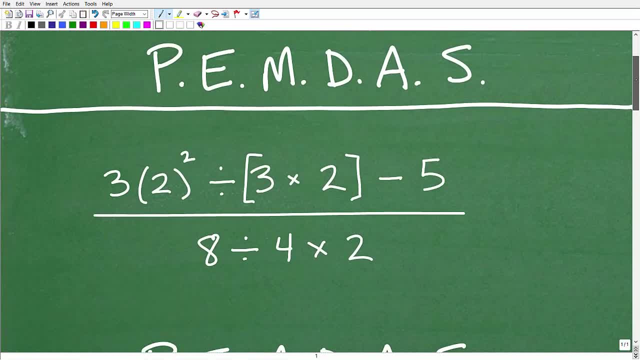 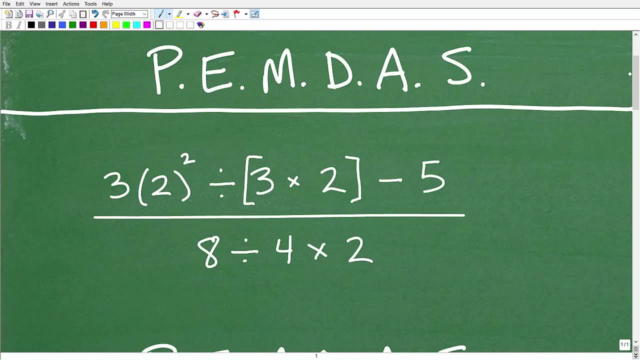 All right, So let's get into the problem. All right, So here is the problem. OK, And I'm not going to recite it, but here it is, And I wouldn't. I suggest that all of you out there, you know, pause the video and just go ahead and knock this problem out. 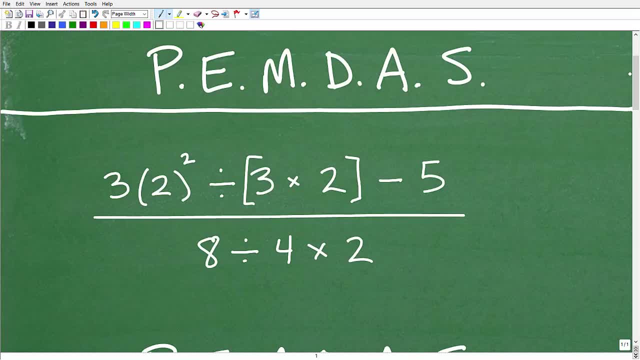 OK, see if you can do it on your own, Fully simplified. Don't use your calculator, just a pencil and a piece of paper. Again, if you're watching this video, you're certainly interested in the order of operations. That either means that you're learning it for the first time. 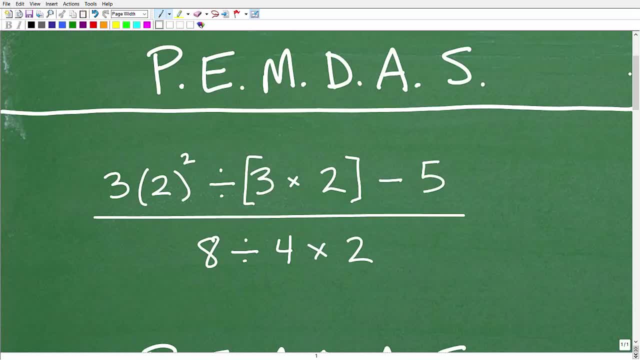 You don't know what you're doing, or maybe you're like struggling with it. OK, so go ahead and and try this problem, even if you're not sure what you're doing, because you might very well be making one of the common errors on what you're talking about. 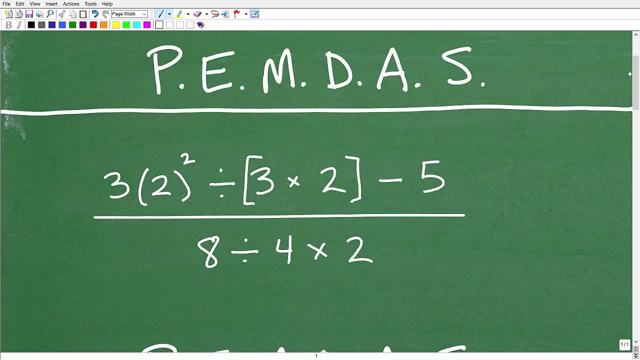 And again, I'm going to highlight these errors and these, these common confusions, if you will, so you can avoid them. All right, So let's get into the problem, But before we do that, let's talk about this: PEMDAS Right. 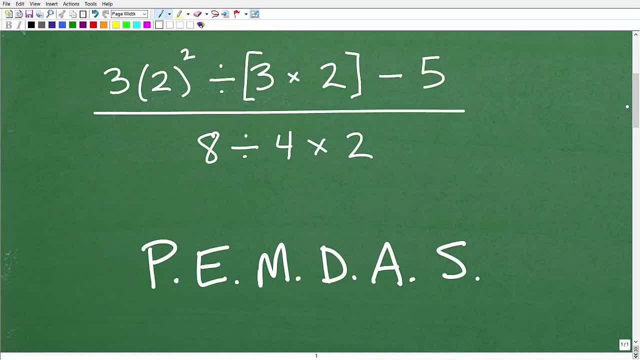 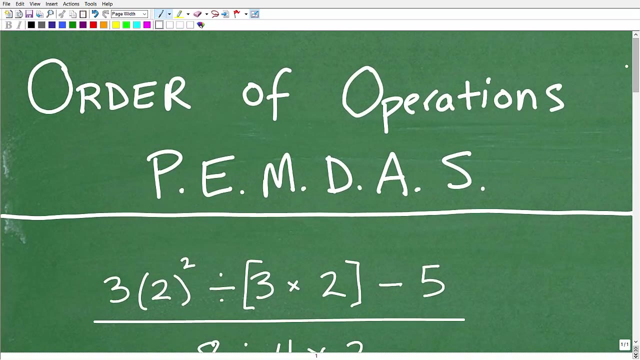 So PEMDAS is our kind of our. it's our guide. OK, It's the instructions On how to apply the order of operations. Now, what does this mean? OK, let's go back up here real quick. Order of operations. 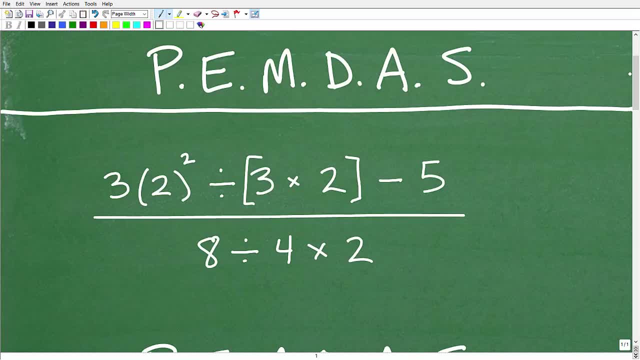 OK, see if you can do it on your own, Fully simplified. Don't use your calculator, just a pencil and a piece of paper. Again, if you're watching this video, you're certainly interested in the order of operations. That either means that you're learning it for the first time. 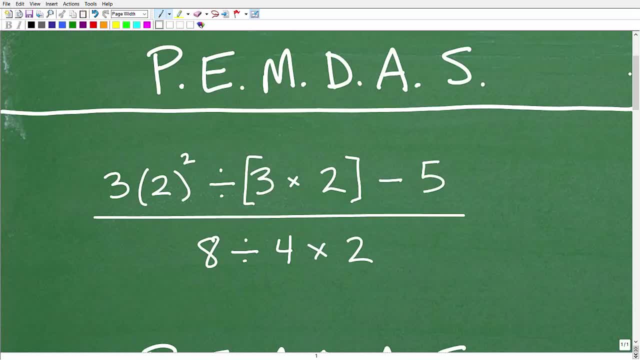 You don't know what you're doing, or maybe you're like struggling with it. OK, so go ahead and and try this problem, even if you're not sure what you're doing, because you might very well be making one of the common errors on what you're talking about. 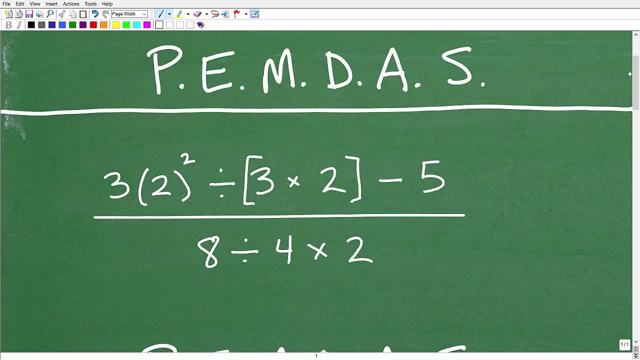 And again, I'm going to highlight these errors and these, these common confusions, if you will, so you can avoid them. All right, So let's get into the problem, But before we do that, let's talk about this: PEMDAS Right. 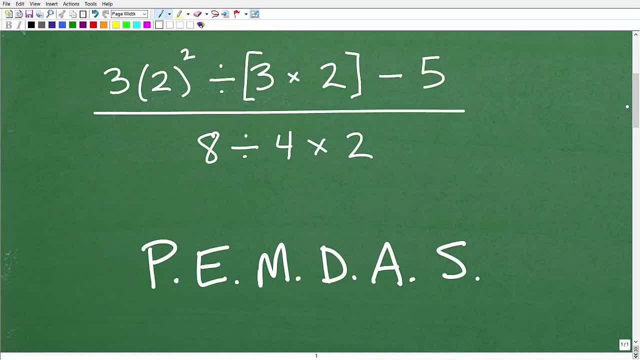 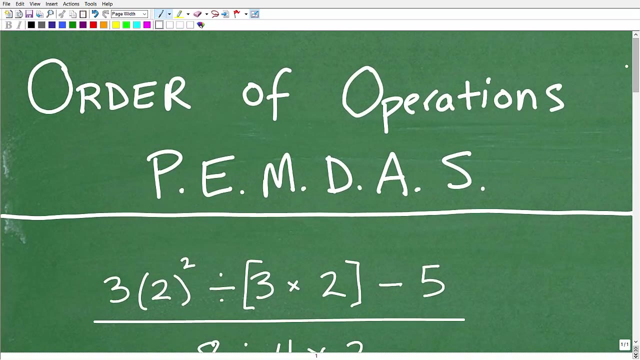 So PEMDAS is our kind of our. it's our guide. OK, It's the instructions On how to apply the order of operations. Now, what does this mean? OK, let's go back up here real quick. Order of operations. 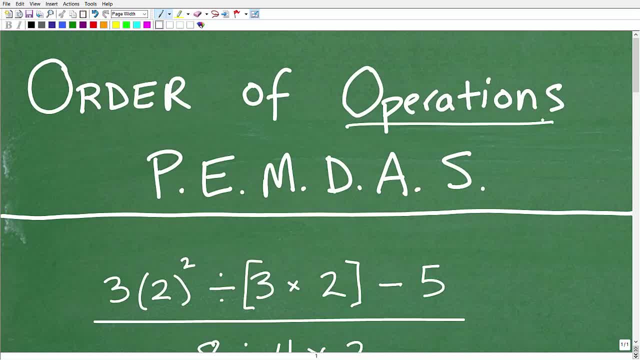 This means something right. Well, in mathematics, operations are things like this: addition, subtraction, multiplication, division, powers, things like this. These are example of mathematical operations. These are mathematical operators, OK, And we need to follow a particular order because if you look here, our problem- OK, we have all kinds of things going on. 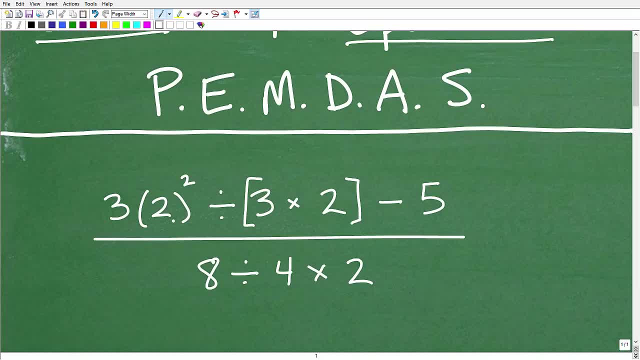 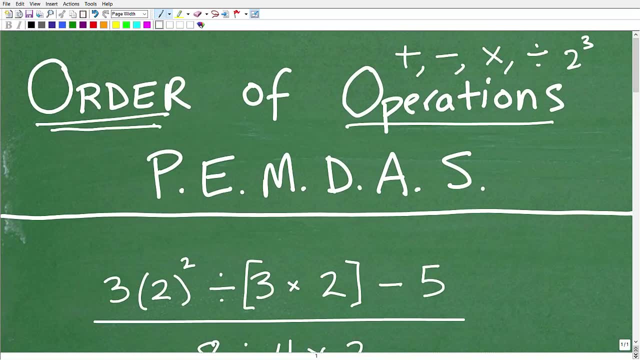 We got multiplication, subtraction, division, powers, fractions. you know it's like: well, what do we do first? OK, And if you don't follow the correct order you're going to get the wrong problem. So order definitely makes a difference. 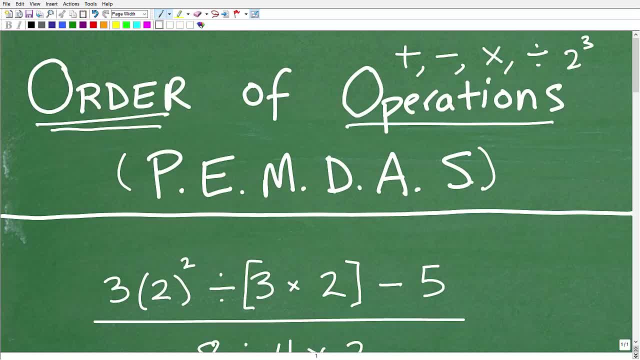 And PEMDAS is our directions. OK, It is the order we want to follow. OK, But just to kind of emphasize this, there is a very specific order to simplifying expressions that have all these mathematical operators, some or all. OK, All right. 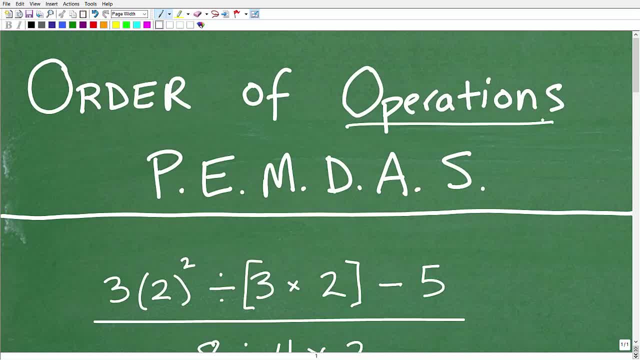 This means something right. Well, in mathematics, operations are things like this: addition, subtraction, multiplication, division, powers, things like this. These are example of mathematical operations. These are mathematical operators, OK, And we need to follow a particular order because if you look here, our problem- OK, we have all kinds of things going on. 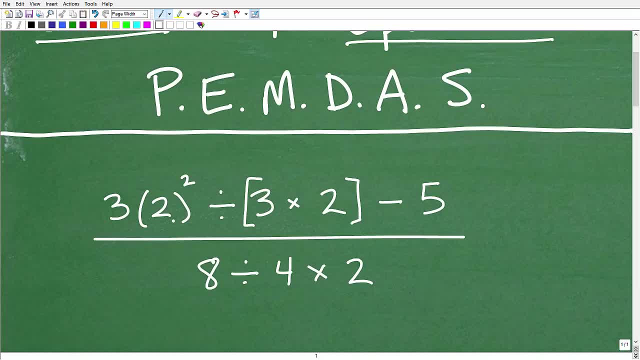 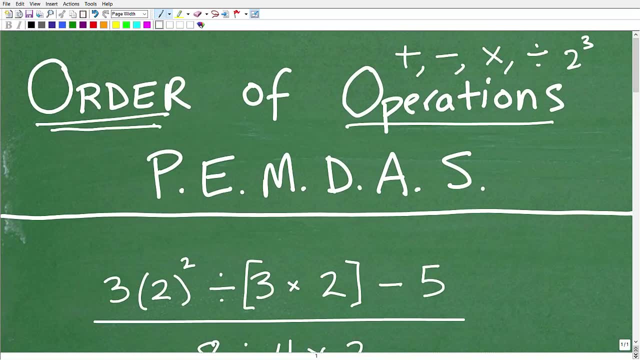 We got multiplication, subtraction, division, powers, fractions. you know it's like: well, what do we do first? OK, And if you don't follow the correct order you're going to get the wrong problem. So order definitely makes a difference. 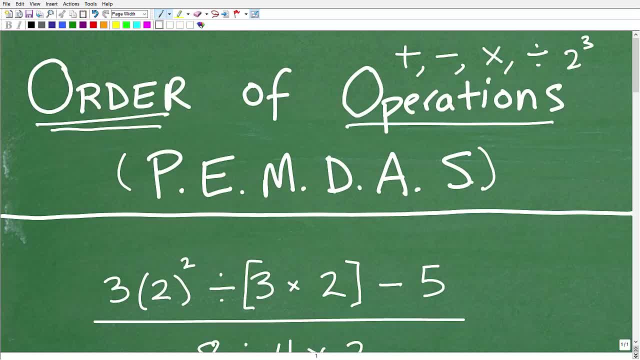 And PEMDAS is our directions. OK, It is the order we want to follow. OK, But just to kind of emphasize this, there is a very specific order to simplifying expressions that have all these mathematical operators, some or all. OK, All right. 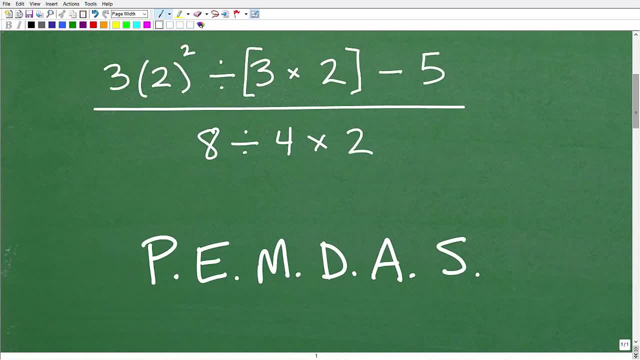 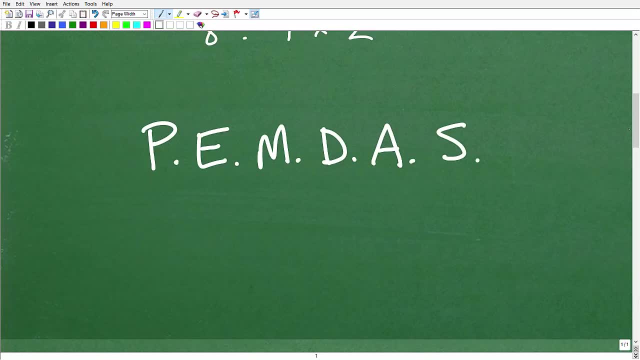 So let's get down to this PEMDAS here again, All right. So let's just review what this means. Now, some of you might know this. There's all kinds of cute little phrases out there. Please excuse my dear Aunt, Sally is one, probably one of the most famous. 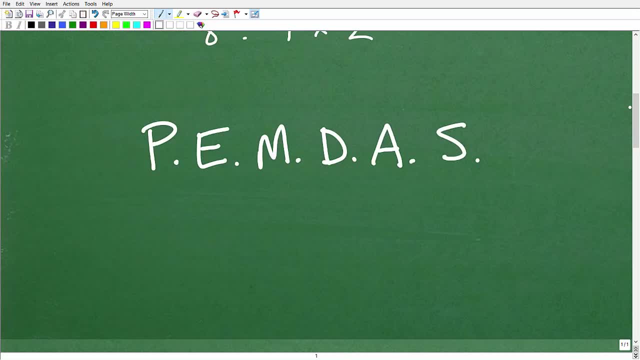 They got probably learned that many, many, many decades ago when I was learning the order of operations. But your teacher might use another one. But almost everyone has some sort of mnemonic. OK, So we don't have one, Go ahead and use. Please accuse my dear Aunt Sally Sue. 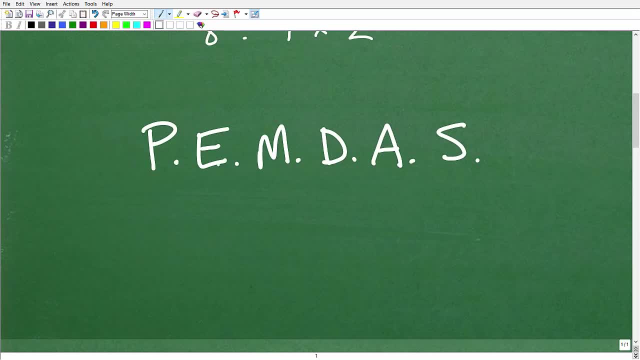 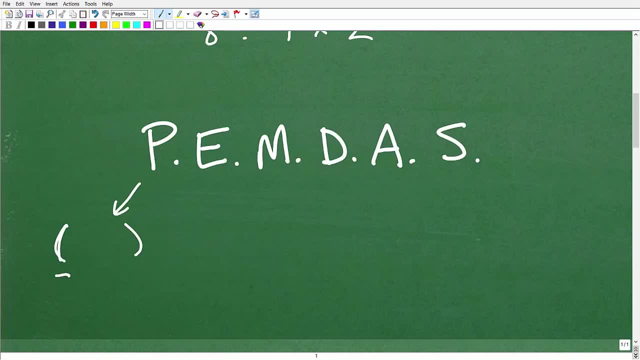 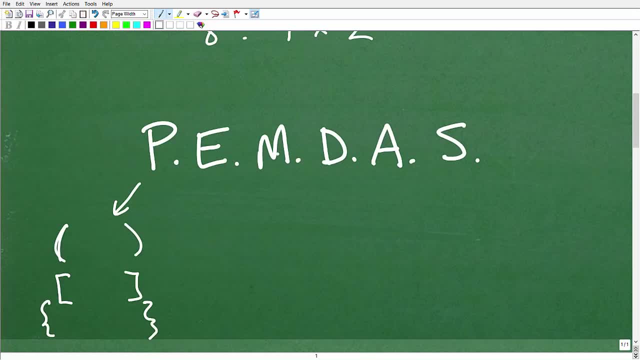 these brackets. these are called grouping symbols. so this little PEMDAS is telling us what to start first. we're going to look for these guys first, and then we're going to kind of go from left to right. we're going to just check to see these operators. so this is our order. okay, we're going. 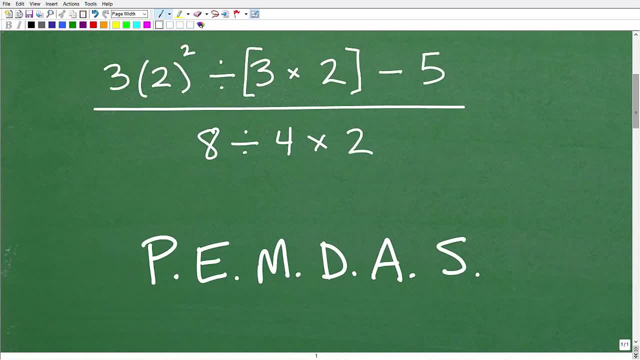 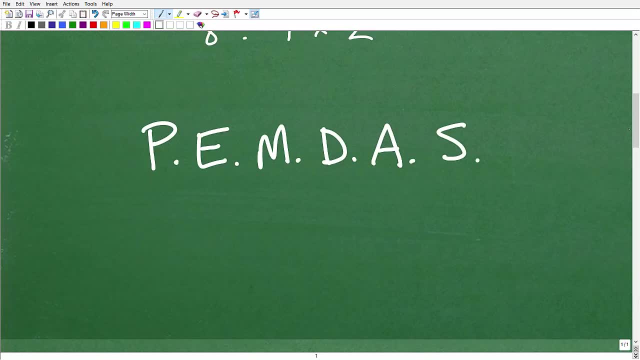 So let's get down to this PEMDAS here again, All right. So let's just review what this means. Now, some of you might know this. There's all kinds of cute little phrases out there. Please excuse my dear Aunt, Sally is one, probably one of the most famous. 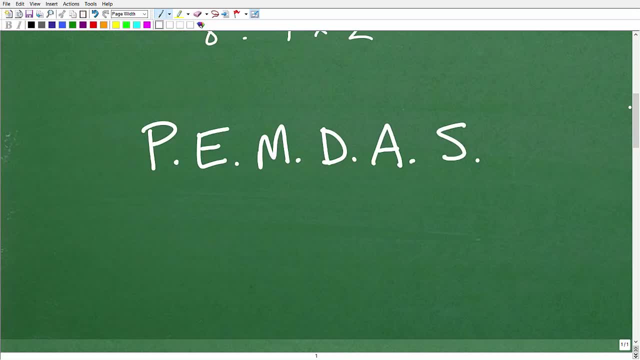 They could probably learn that many, many, many decades ago when I was learning the order of operations. But your teacher might use another one. But almost everyone has some sort of mnemonic. OK, So we don't have one? Go ahead and use, Please. 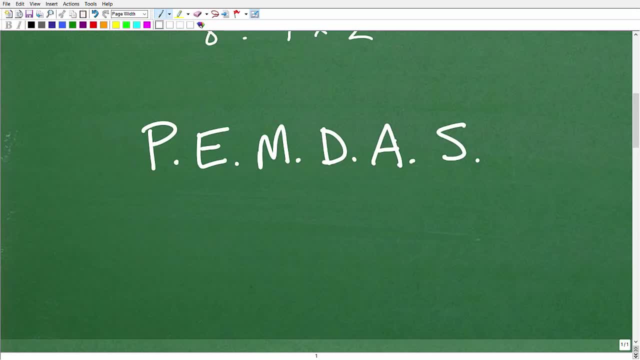 Excuse my dear Aunt Sally. So remember PEMDAS. OK, Now, what does this stand for? Well, P, let's just do a quick review. Stands for parentheses. OK, so you're going to do things. we want to do things first. 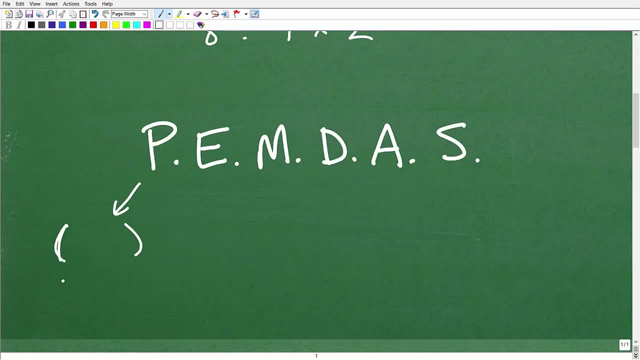 So you're going to do things. We want to do things first. first, okay, that are in parentheses or brackets, or even, like these little squiggly kind of guys, these brackets. these are called grouping symbols. so this little pemdos is telling us what to start. 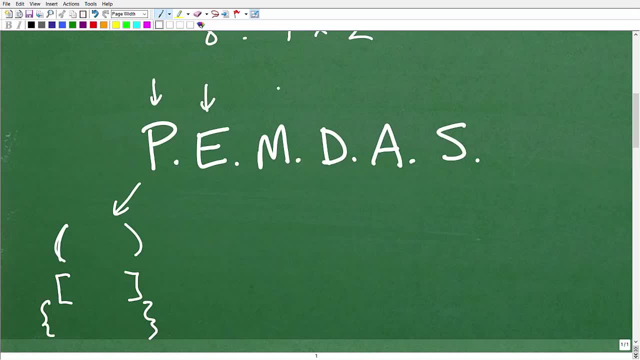 first, we're going to look for these guys first, and then we're going to kind of go from left to right. we're going to just check to see these operators. so this is our order. okay, we're going to start here and we're going to proceed this way, kind of go through a little checklist. okay, so p. 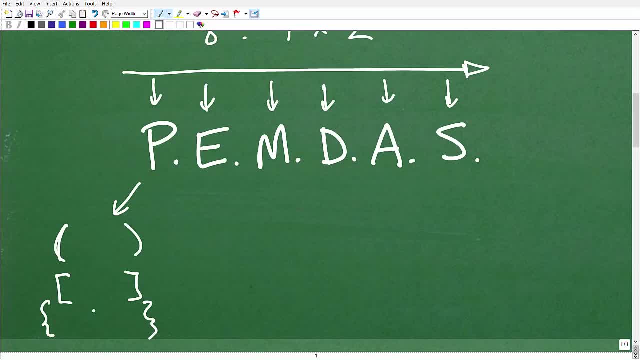 is everything inside parentheses. okay, we're going to be looking for parentheses or brackets, or little squiggly brackets, and we're going to do everything inside them. okay, now, after we've kind of done that, and again there's a lot of variations, different type of practice, problems. 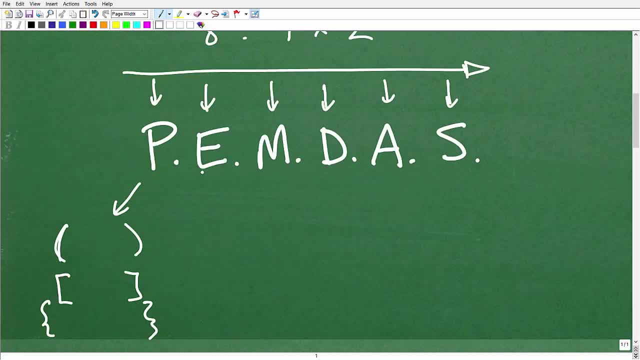 involved in here. this is just a basic overview of this pemdos. okay, so, e what does e stand for? okay, well, e is really a stands for exponent, so you kind of think of it like this two cubed, this little e is an exponent, but really just think of e as powers. okay, we're going to do. 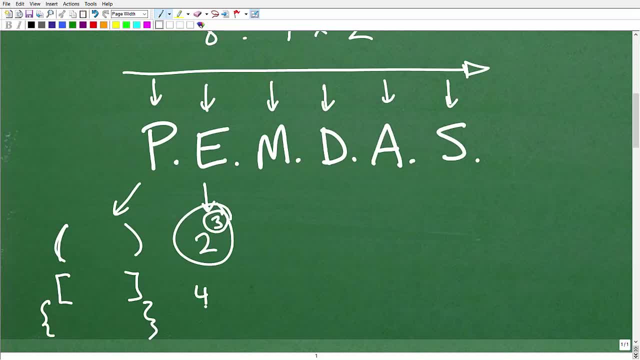 any powers next. okay, so like two cubed or four squared things like that. that's what e stands for. okay, we're going to do powers next, and then we have m and d. so m and d, this is multiplication and this is division. okay, let's just go and put the rest in here. this is addition. 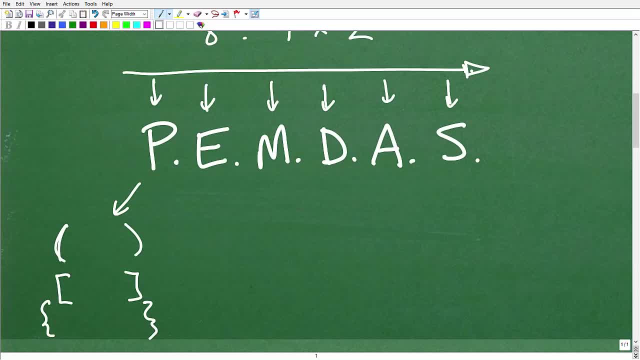 to start here and we're going to proceed this way, kind of go through a little checklist, okay. so p is everything inside parentheses. okay, we're going to be looking for parentheses or brackets or little squiggly brackets, and we're going to do everything inside them. okay, now, after we've, 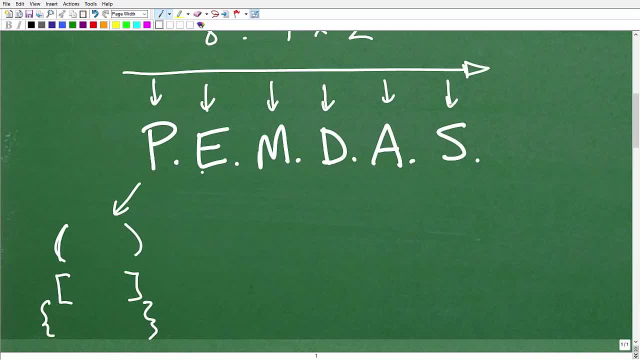 kind of done that and again there's a lot of variations, different type of practice, problems involved in here. this is just a basic overview of this PEMDAS. okay. so, e what does e stand for? okay, well, e is really a stands for exponent, so you kind of think of it like this: 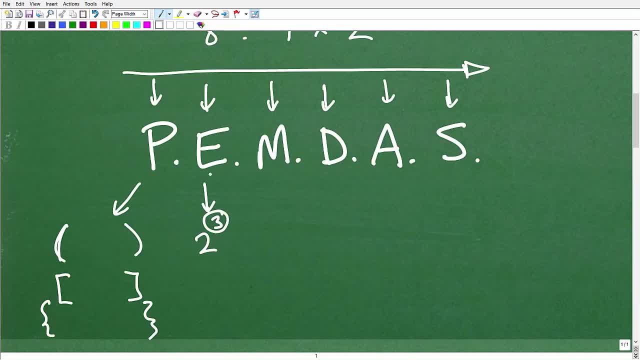 two cubed. this little e is an exponent, but really just think of e as powers. okay, we're going to do any powers next. okay, so like two cubed or four squared things like that. that's what e stands for. okay, we're going to do powers next. and then we have m and d. so m and d- this is multiplication. 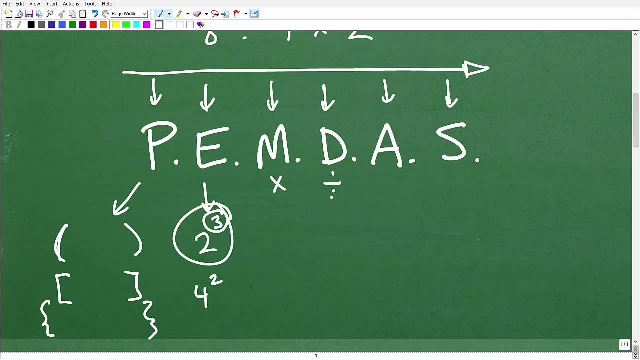 and this is division. okay, let's just go and put the rest in here: this is addition and this is subtraction. now, this is probably uh, one of the big areas where students get confused on PEMDAS is we need to look at multiplication and division and addition and subtraction kind of as little. 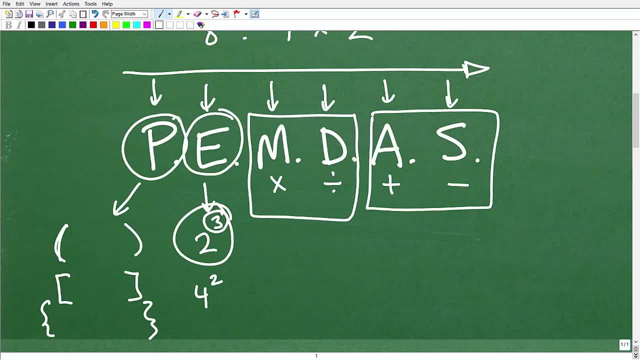 bundles here. so we have p by itself, e by itself, now multiplication and division. so what we're going to do here is we're going to multiply okay, then divide, or we're going to divide, then multiply, but the difference is that in multiplication I'm dividing, and dividing I'm going to divide. 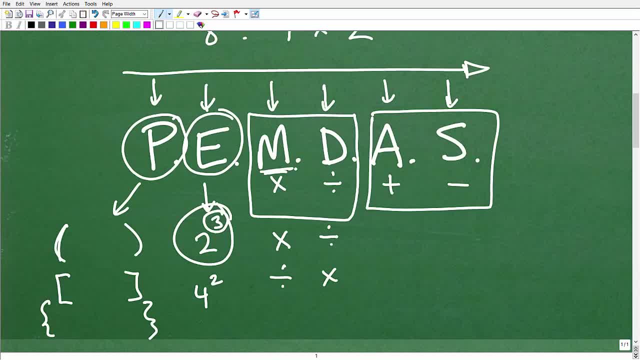 by multiplying, okay. so I'm taking the expression here and I'm taking the expression here and I'm dividing by multiplying a fraction, taking the every single fraction into a Roman form and doing multiple subscriptions. so, as I said, you want to do some multiplication, do multiplication stage. okay, because that's great. but what you're doing is you're not just going. to divide you. you want to gomap big elementary five learning guys, but you want to divide what's in you by dividing. so does the multiplication day okay, but you can change that. it's different if you change it like um. so divide by multiplying makes a big difference between right division. 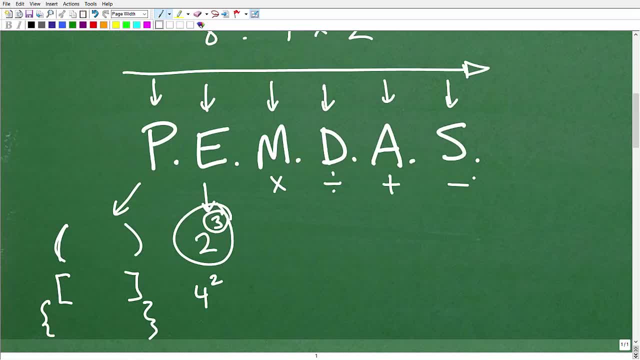 and this is subtraction. now, this is probably. uh, one of the big areas where students get confused on pemdos is we need to look at multiplication and division and addition and subtraction, kind of as little bundles here. so we have p by itself, e by itself, now multiplication and division. so what we're? 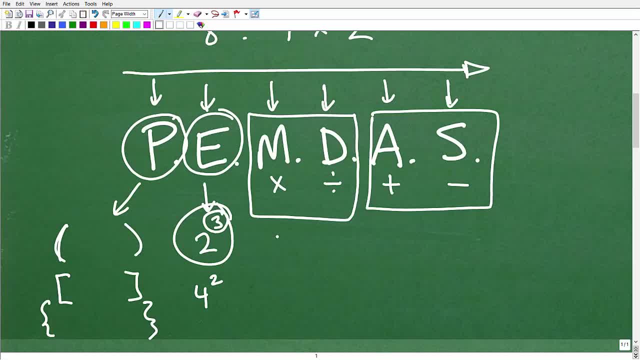 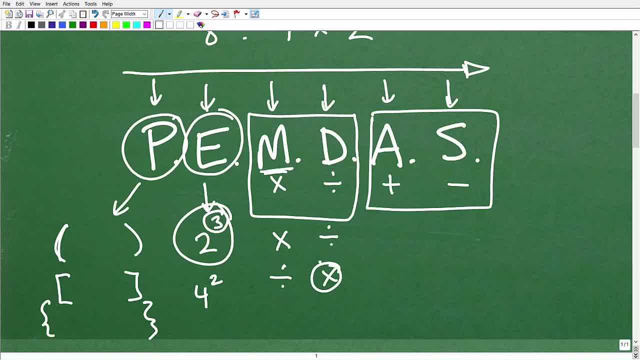 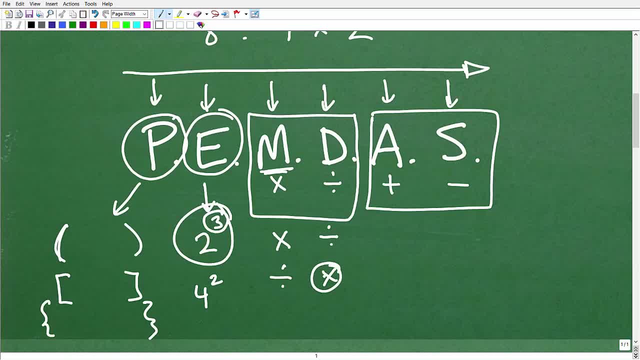 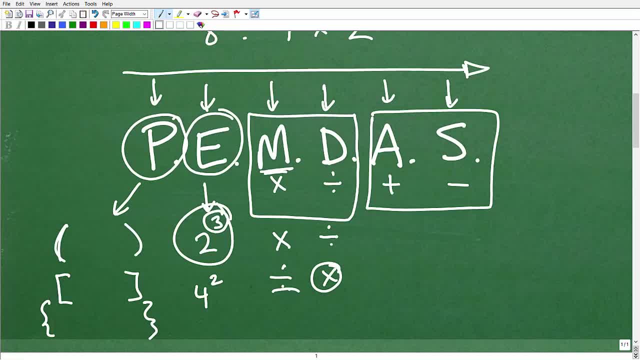 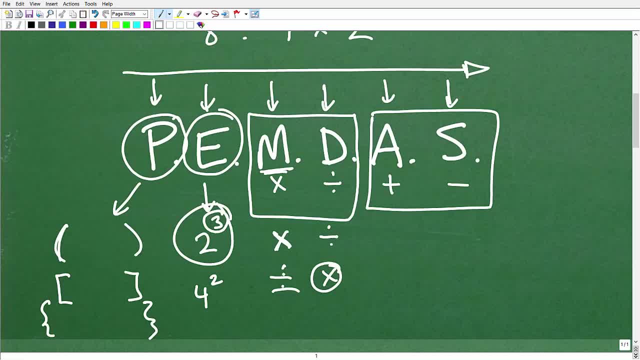 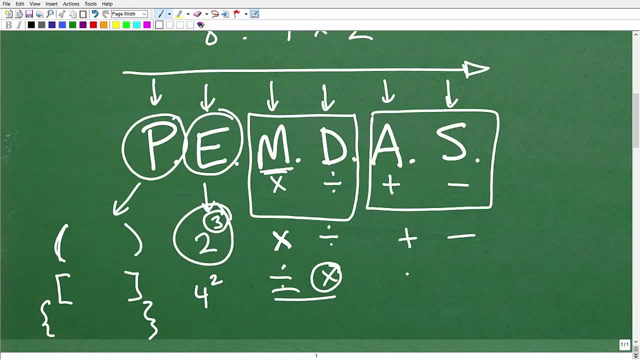 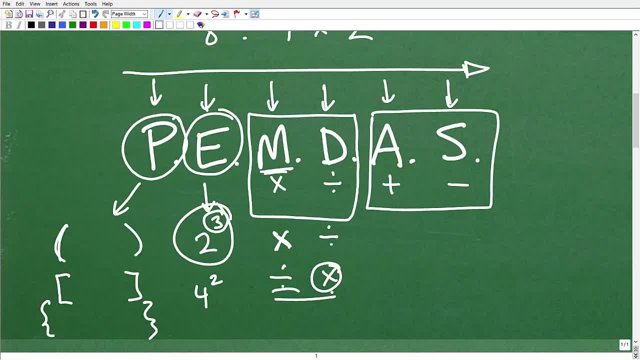 right or left division, and if you divide by multiplying, you're just separate. well, you're somehow subtracting. if you see division and then multiplication, then that's what you're going to do. and same thing applies for a and s addition and subtraction. you're going to do addition or subtraction, or 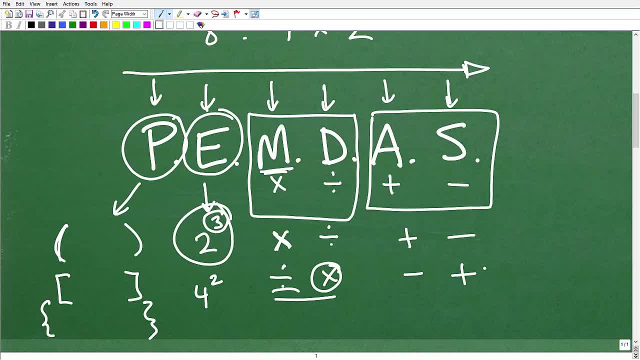 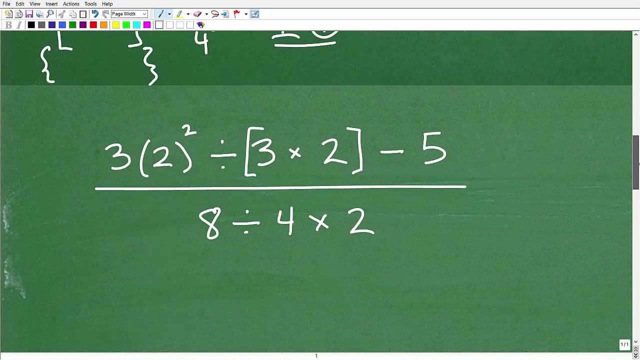 subtraction or addition, whatever you see first, from left to right. okay, so hopefully this has kind of cleared up a lot of- uh, your confusion, if you had any, or strengthen your understanding of pymnos. now let's get to the problem here, and so we can kind of see what's going on. now we have 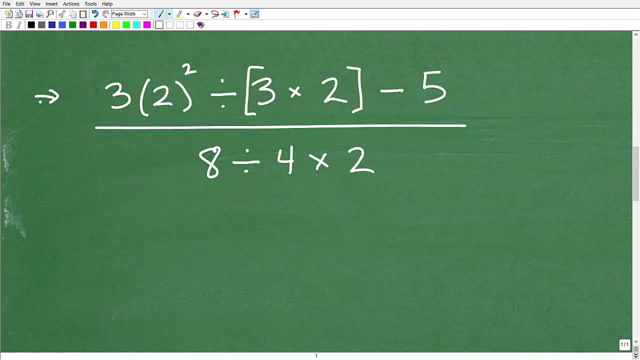 one big gold fraction. right, we have this numerator and this denominator. so what you want to do, the fraction bar in and of itself is kind of like a grouping symbol. so what you want to do is work independently of both the numerator and denominator, in other words, simplify the 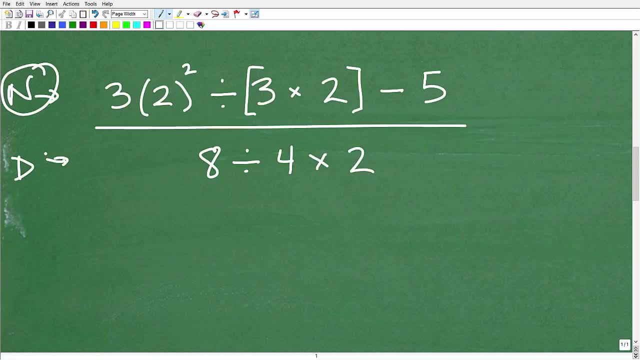 numerator down to one value and then work on the denominator, simplify that down to one value and then you can kind of simplify from there. okay, so you never want to kind of intermingle your work, so you can kind of depending on your um, your skill level, or your, your practice. 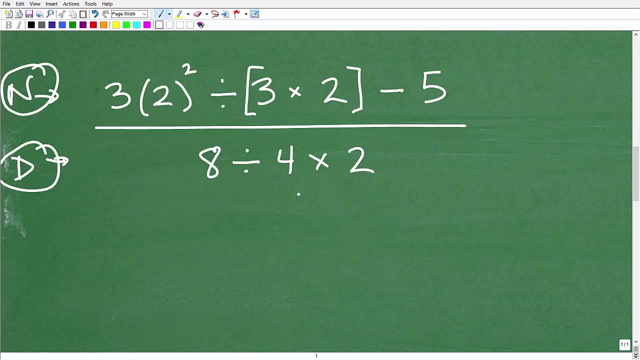 you can do more than one step at a time. i would suggest not doing any more than, say, two steps at a time. okay when you're working a problem down, but whatever you're doing, make sure you show your work so your teacher can follow and you can kind of review and make sure you did everything correct. 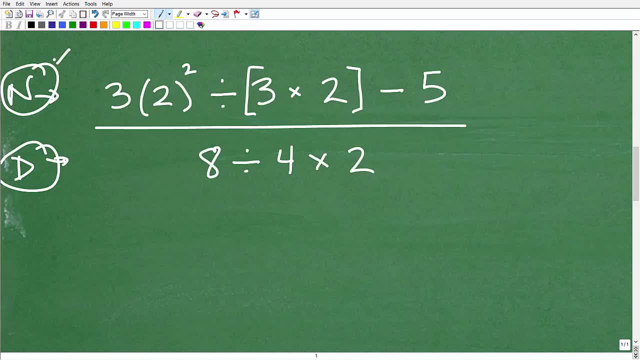 okay. so, with that being said, let's go ahead and just focus in on the numerator for now. okay, so we'll deal with the denominator here in a second. so let's take a look at the numerator. and we're using pemdos, okay, so if you want to write that down, go ahead, and i'm not going to bring 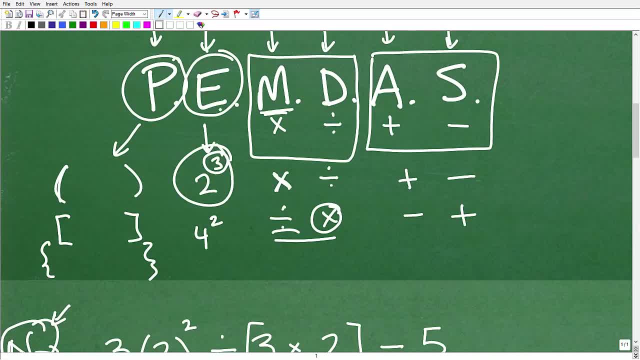 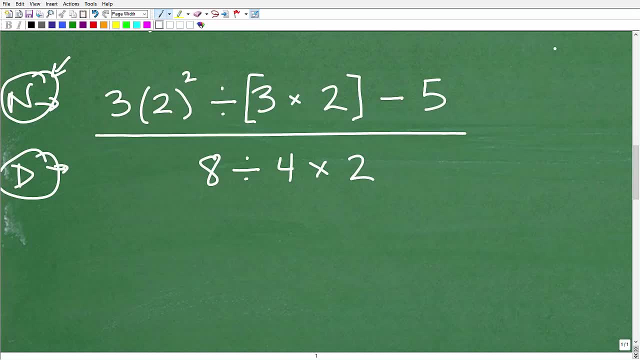 it down with us all the time, but put that down on your piece of paper to the side here so we can just kind of use it as a guide. so the first thing is: i'm looking- well, let me just do it here- what the heck? p-e-m-d-a-s? so i'm focused in on p, okay, 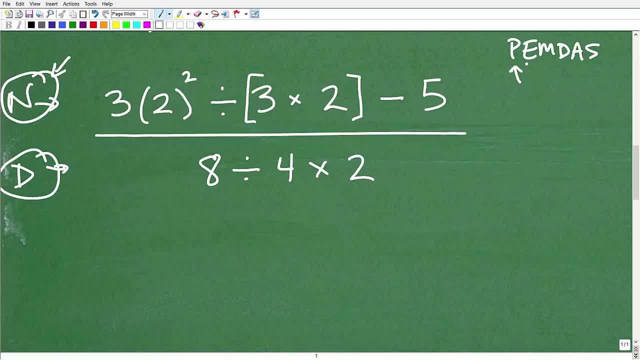 so are there any parentheses? yes, there are. okay, remember parentheses. brackets we call grouping symbols. so here, right here, this part of the problem r is a pair of brackets, so that indicates that we have to do everything inside those brackets first. so let's go ahead and do that. 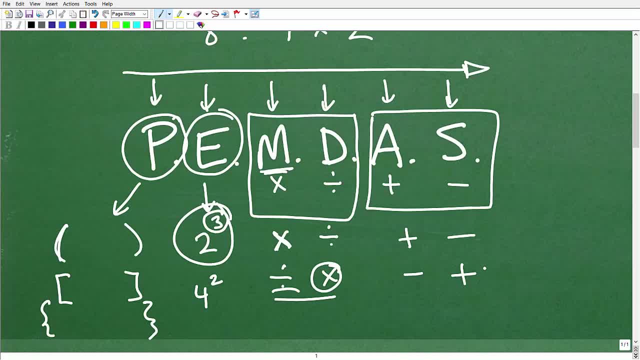 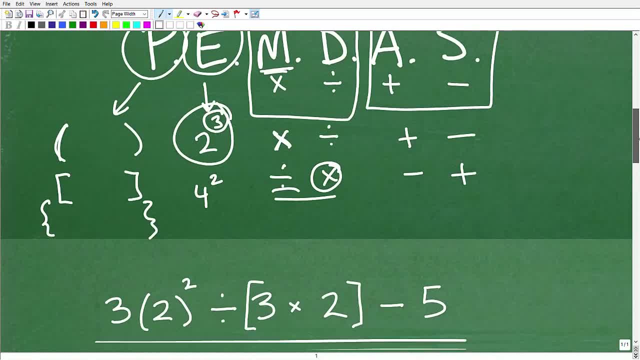 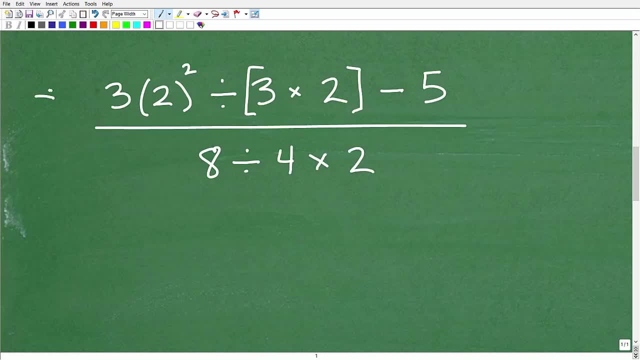 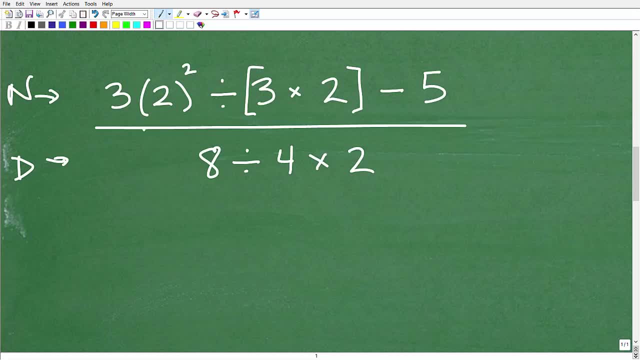 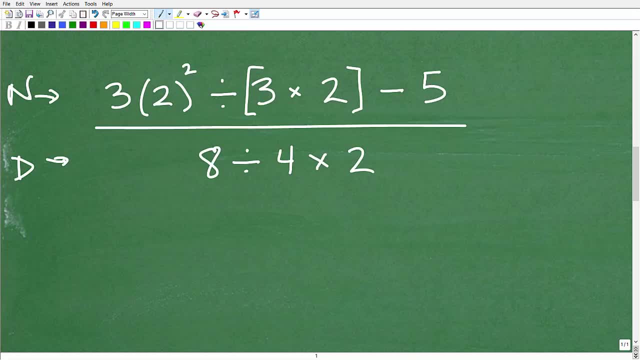 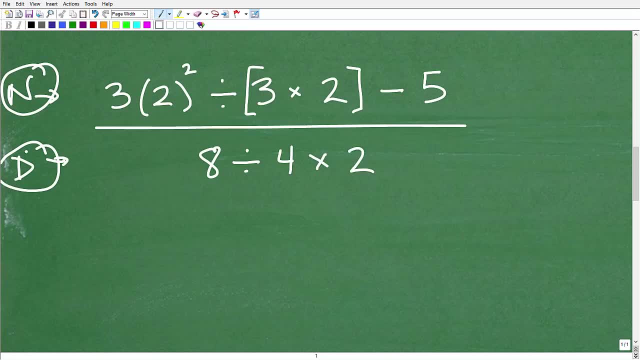 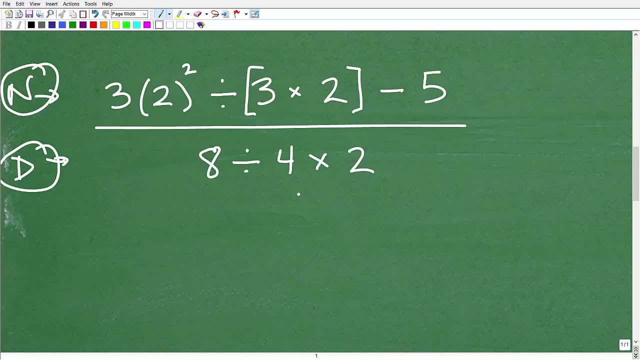 intermingle your work So you can kind of depending on your skill level or your practice, you can do more than one step at a time. I would suggest not doing any more than, say, two steps at a time. okay, when you're working a problem down, But whatever you're doing, make sure you show your. 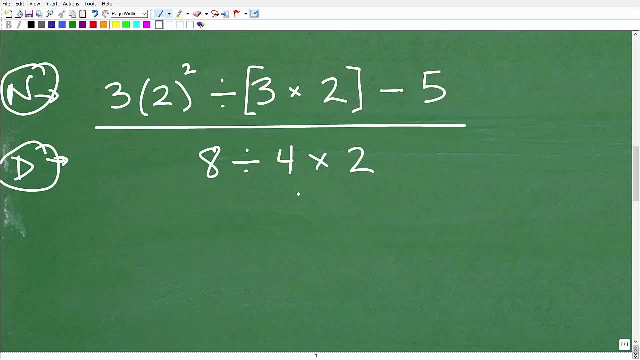 work, so your teacher can follow and you can kind of review and make sure you did everything correct, okay? So, with that being said, let's go ahead and just focus in on the numerator for now. okay, So we'll deal with the denominator here in a second. So let's take a look at the numerator. 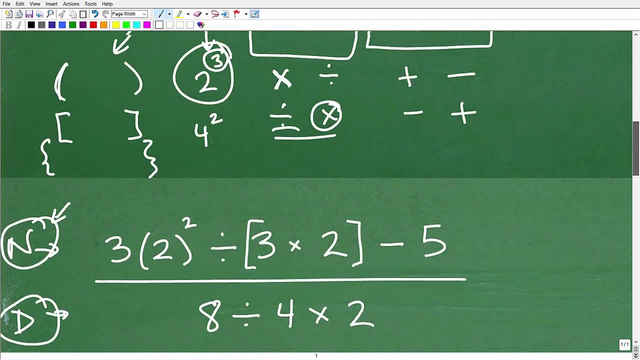 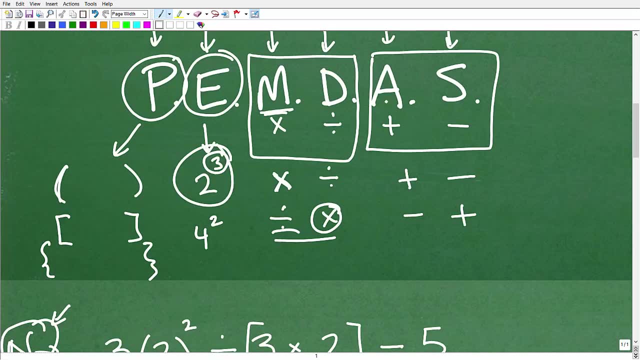 and we're using PEMDAS, okay. So if you want to write that down, go ahead, and I'm not going to bring it down with us all the time, but put that down on your piece of paper to the side here so we can just kind of use it as a guide. So the first thing is I'm looking. well, let me just 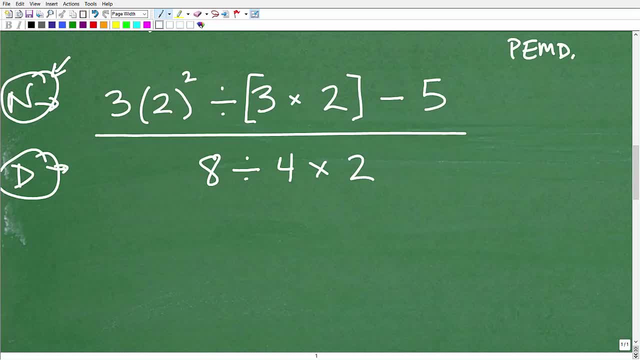 do it here. What the heck? P-E-M-D-A-S. So I'm focused in on P, okay, OK. so are there any parentheses? Yes, there are. OK, remember parentheses, brackets we call grouping symbols. 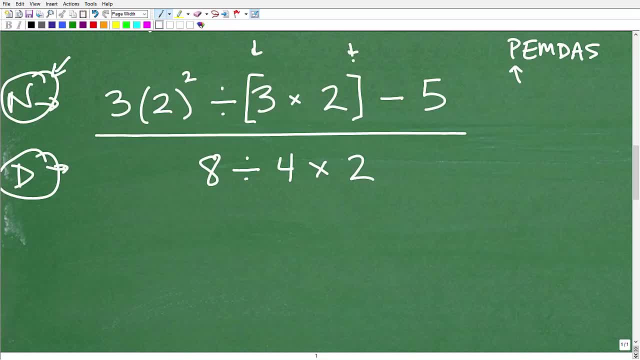 So here, right here, this part of the problem is a pair of brackets, So that indicates that we have to do everything inside those brackets first. So let's go ahead and do that, And the way I'm going to show that is I'm just going to simply rewrite the numerator. 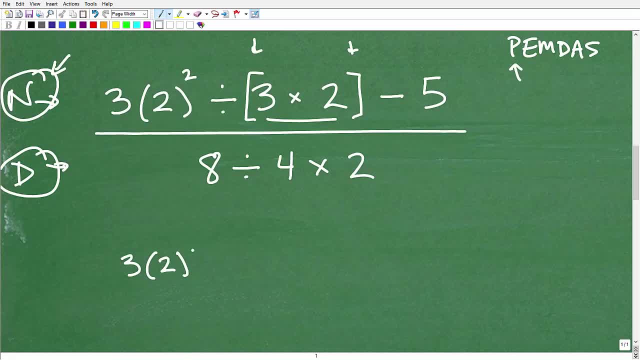 OK. three times two squared. Be very careful here. Divided by bracket. Now three times two. I'm going to do what's inside the parentheses. That is six. OK minus five, All right, So go ahead and rewrite the denominator. 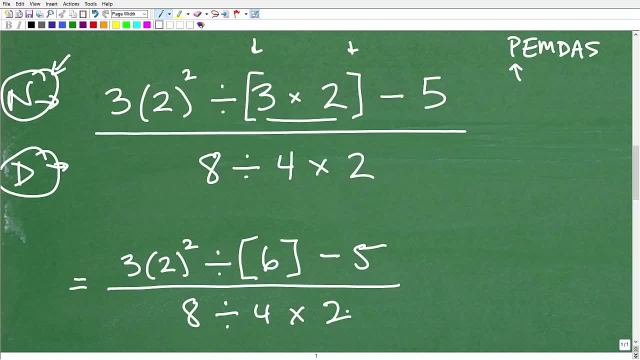 Eight divided by four times two. Now you're like boy: that's a lot of writing. I can take a couple of steps at once. Again, this is where students get in trouble in math. They become impatient or like: all right, I'm going to do this step. 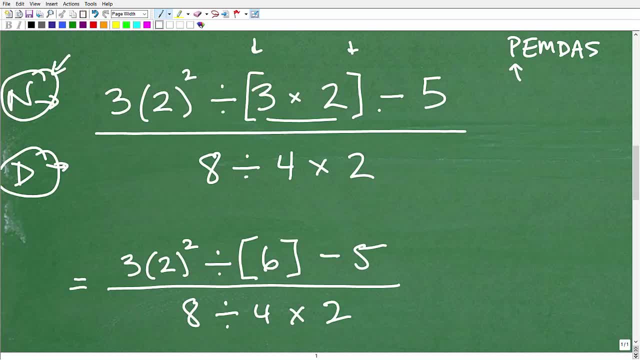 that step and this step and this step, And it's a noble, you know kind of gesture. You're like, hey, I'm going to save time and space on my paper, But it more often than not it messes students up. OK, take a step, maybe two at most. 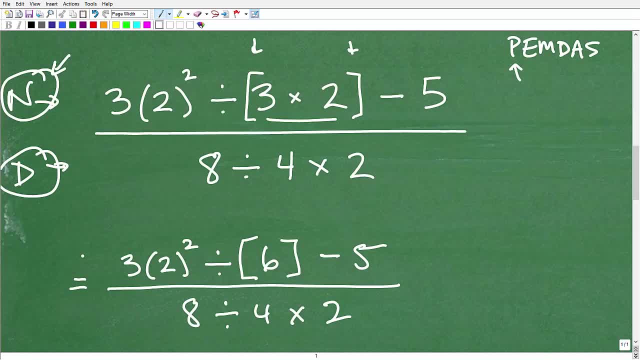 OK, look to see after you're done. OK, look at your work. Make sure you copied the problem down correctly. So three times two squared, Divided by three times two, is six. That was I supposed to do. Minus five Eight, divided by four times two: Boom, I'm happy. 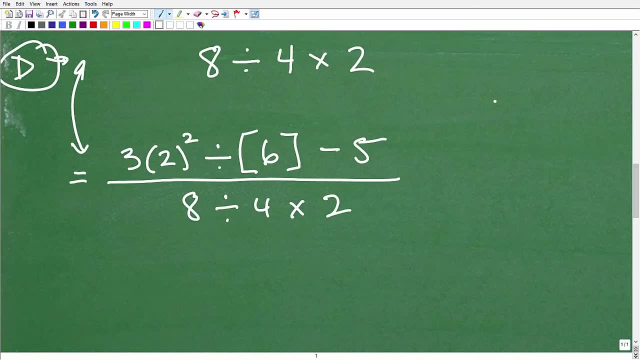 OK, so now let's continue to focus on the numerator And let me write our little pen and dots here. All right, So are there any more parentheses? No, So now there's, there's this bracket. here You're saying: well, there's the brackets. 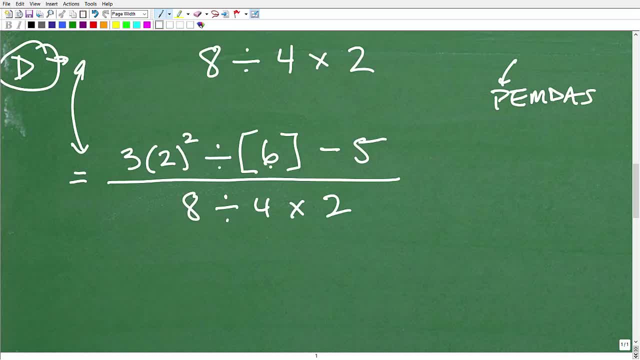 Yeah, but really, when there's nothing, there's nothing else to do. You can simply just drop those brackets. We'll just leave there for a second, But there's no more brackets, So now let's go and check for E. OK, are there any powers? 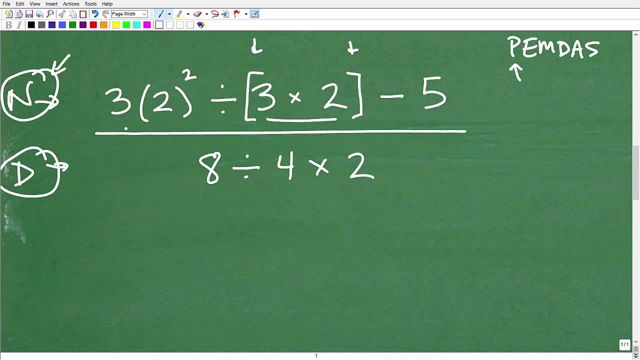 and the way i'm going to show that is: i'm just going to simply rewrite the numerator okay, three times two squared- and be very careful here- divided by bracket. now, three times two. i'm going to do what's inside the parentheses. that is six, okay, minus five. all right, so go ahead and rewrite the denominator eight divided by four times two. 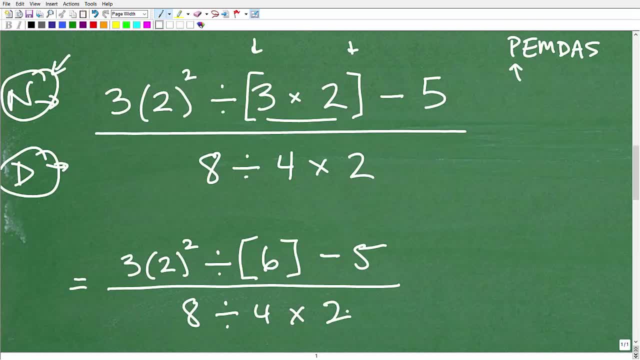 now you're like boy: that's a lot of writing. i can take a couple steps at once again. this is where students get in trouble in math. they become impatient or like, all right, i'm going to do this step, that step and this step and this step. 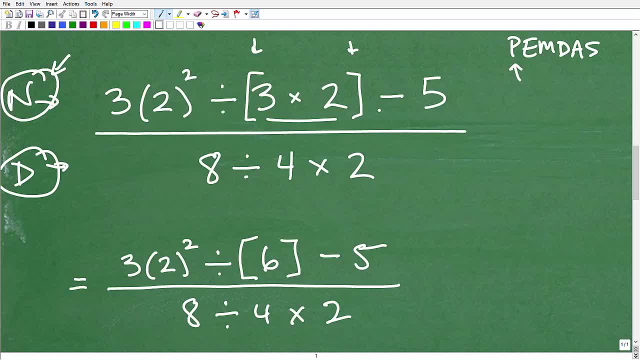 and it's a noble, you know kind of gesture. you're like, hey, i'm going to save time and space on my paper, but it more often than not it messes students up. okay, take a step, maybe two at most. okay, look to see after you're done. okay, look at your work, make sure you copied your. 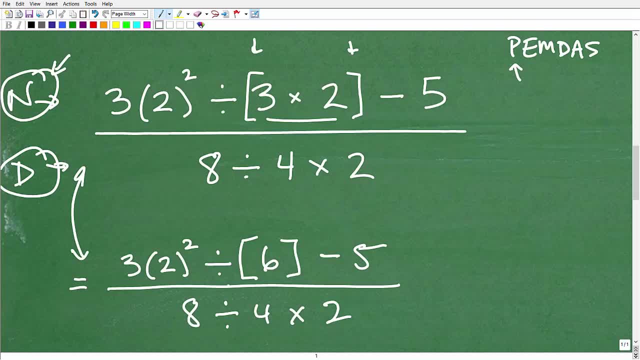 the problem down correctly. so three times two, squared, divided by three times two, is six. that was i supposed to do. minus five, eight divided by four times two: boom, i'm going to do that, okay. so now let's continue to focus on the numerator and let me write our little pindas here. 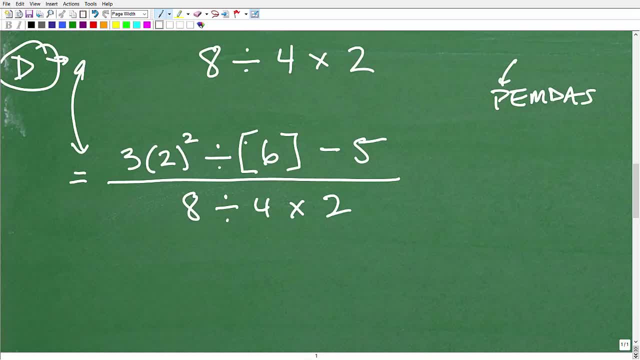 all right, so are there any more parentheses? no, so now there's. there's, uh, this bracket here. you're saying: well, there's the brackets, yeah, but really, when there's nothing, there's nothing else to do. you can simply just drop those brackets, we'll just leave there for a second, but there's no. 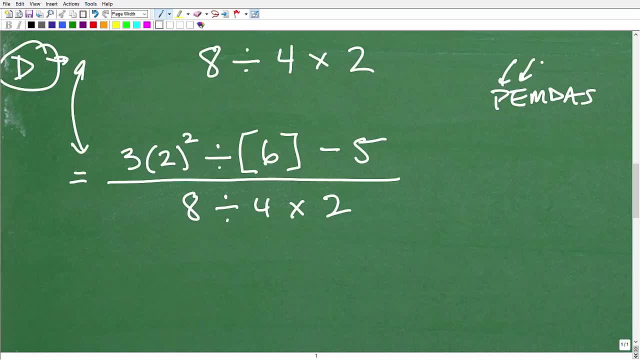 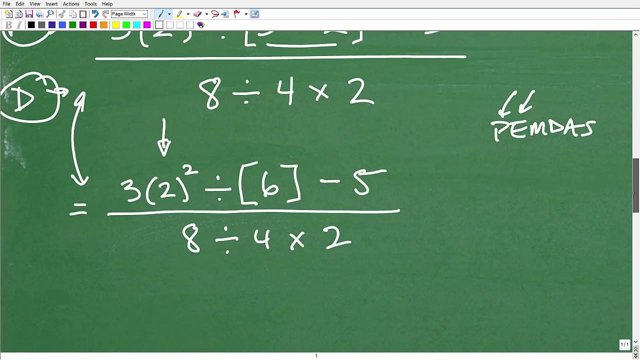 more brackets. so now let's go and check. uh for e. okay, are there any powers? yes, there are powers right here. two squared- okay, now, let me just make sure that i didn't. uh, this problem is two squared, not two cubed. just want to double check. all right, now, this is a real, another big area of confusion. 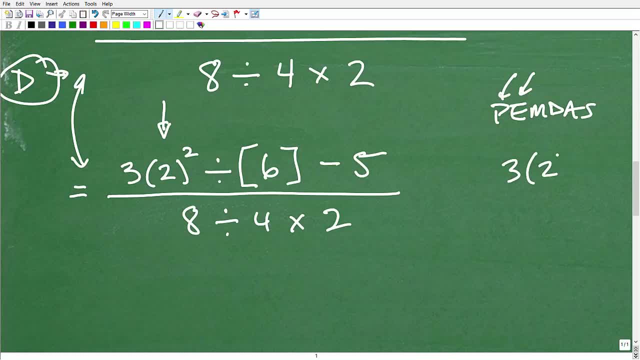 here's the mistake that i would see, uh, thousands of times, uh, through the years as a, as a teacher. um, i would see this mistake. oh, let's do an encounter this: they would go three times. two is six, six square 36. that's what they would do. totally wrong, because they're not doing powers first. okay, 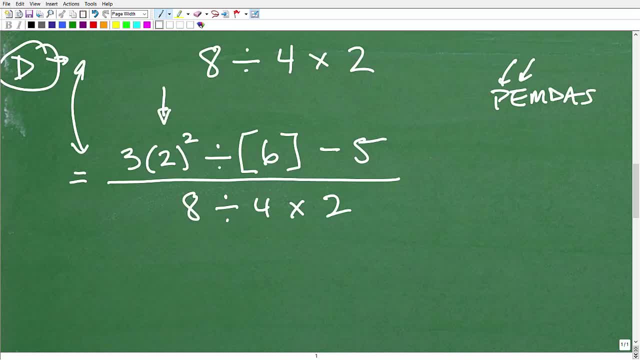 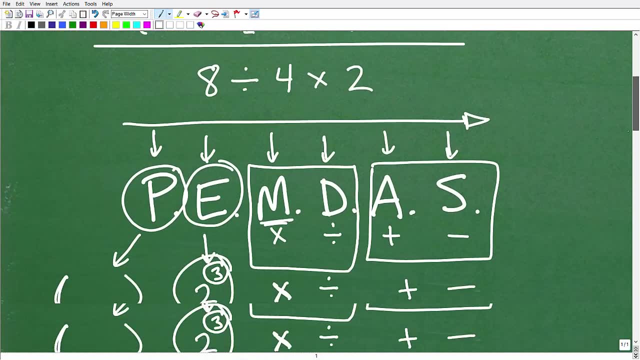 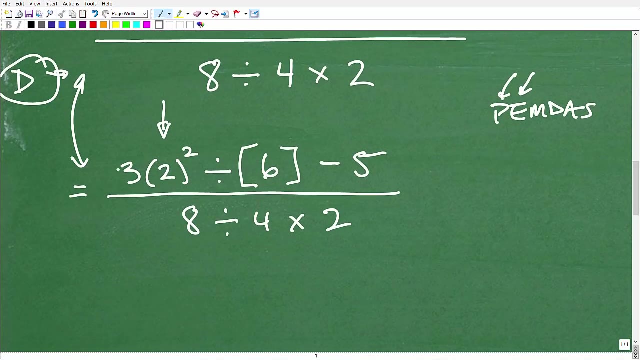 Yes, there are powers. OK, right here. Two squared- OK, Now let me just make sure that I didn't. This problem is two squared, not two cubed. Just want to double check. All right, Now, this is a real. another big area of confusion. 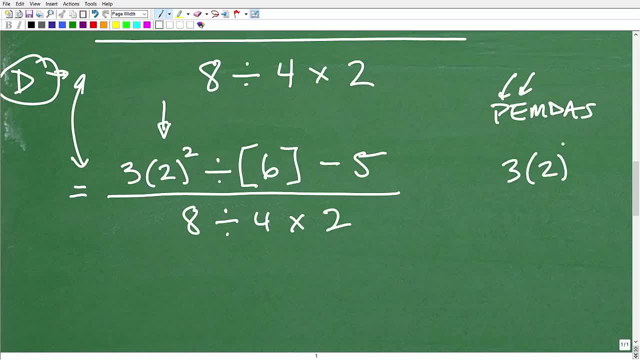 Here's the mistake that I would see thousands of times through the years. as a teacher, I would see this mistake. Oh, let's do an encounter This: they would go three times. two is six, six square thirty six. That's what they would do. Totally wrong, because they're not doing powers first. 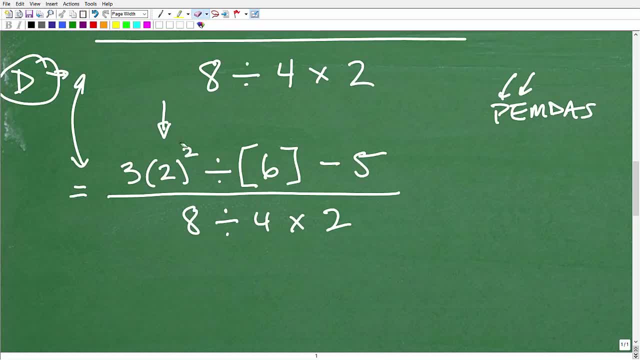 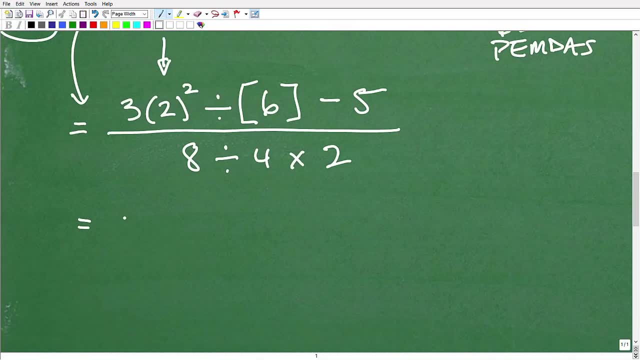 OK, so that's what we got to do. We have to go to square. which is what? Two times two, So that's going to be four. So let's just walk it down like this: Three times four divided, by Now we could just drop this bracket. 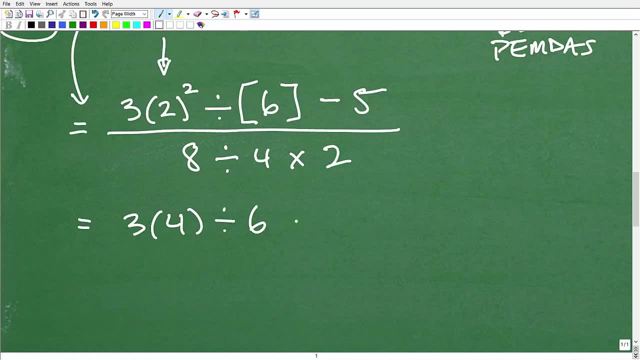 Brackets here. It's a little redundant. There's nothing more to do here. Divided by six minus five over eight. divided by four times two: OK, so we did our exponent, OK. so again, I'm still focused on the numerator. 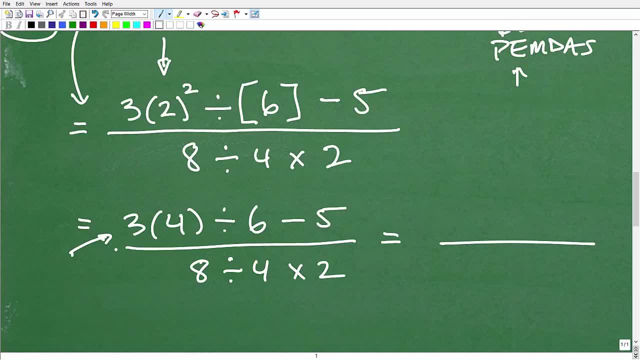 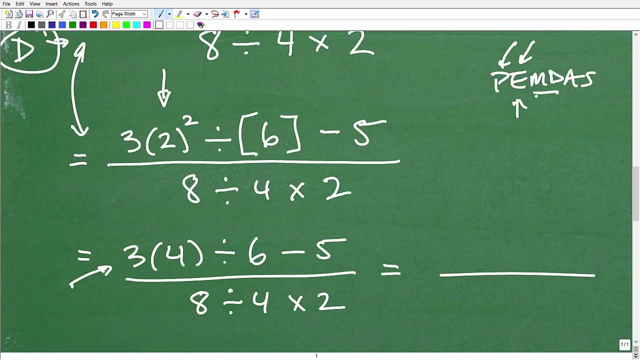 OK, I'm still. I'm focusing here. I'll deal with the denominator in a second. So are there any more powers? I don't see any more powers. Right, We're good there. So now I'm going to look at multiplication and division. 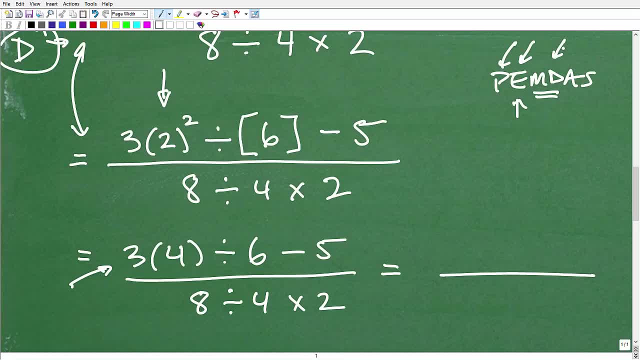 Remember, I'm going to look at this as a bundle, Right? So is there any multiplication and division? Yes, there is. This is multiplication, And then I got division here. So which comes first? OK, well, multiplication comes first from left to right. 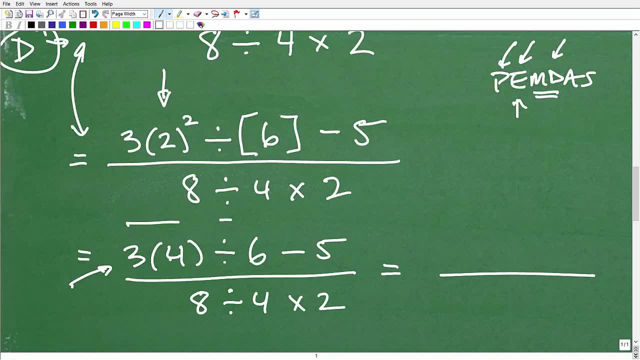 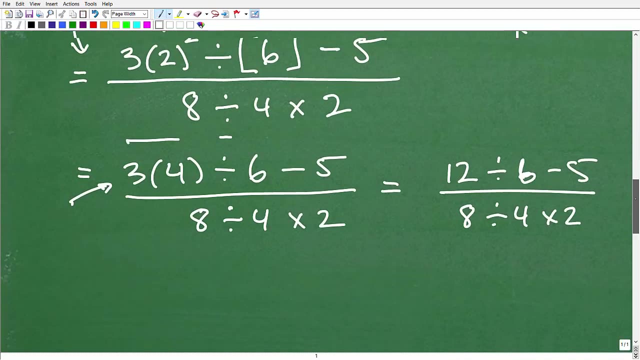 So we're going to go ahead and write that down there. So three times four is twelve divided by six Minus five. Then I have here Eight divided by four times two. OK, so now we're really getting there, Right. 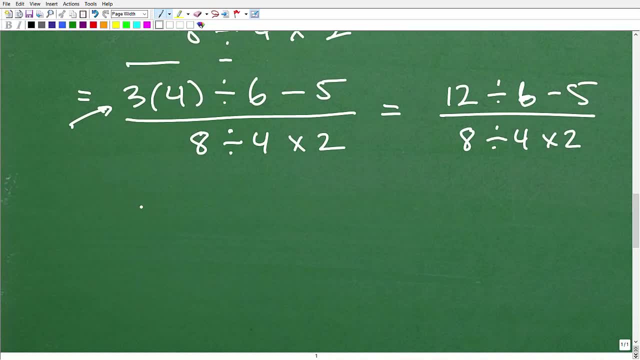 Getting more and more simplified, And I'm going to write this down here: Twelve divided by six minus five, over eight divided by four times two. All right, So let's get our little PEMDAS out again. P-E-M-D-A-S. 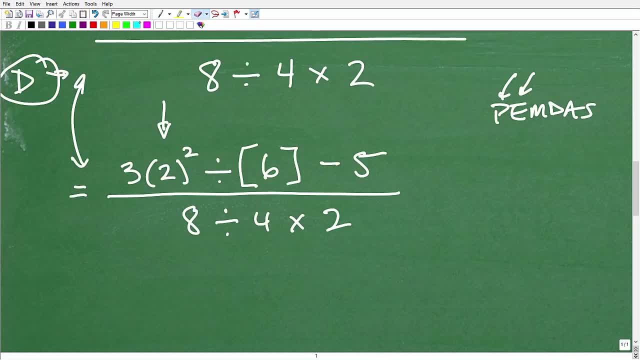 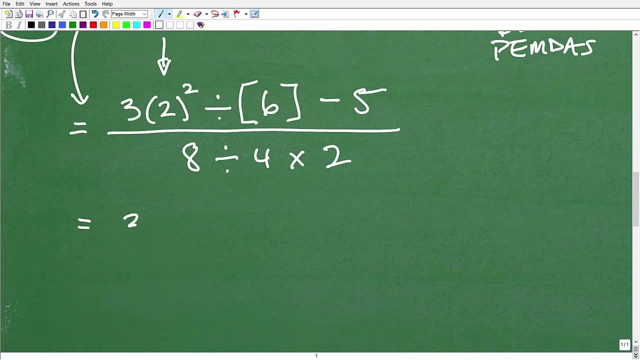 so that's what we got to do. we have to go two square, which is what? two times two? so that's going to be four. so let's just walk it down like this: three times four divided- by now we could just drop this brackets here. it's a little redundant. there's nothing more to do here. divided by six: 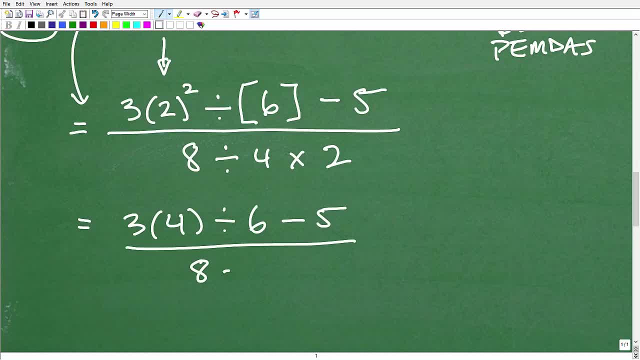 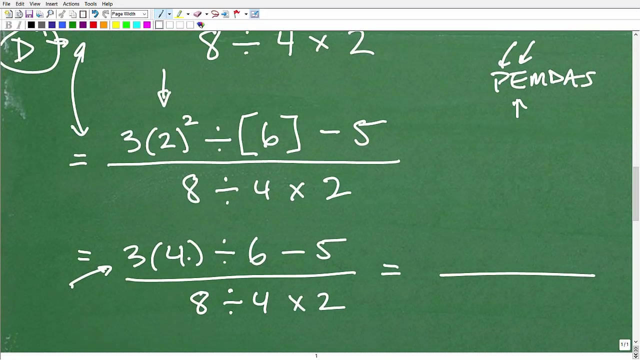 minus five over eight, divided by four times two. okay, so we did our exponent. okay, so again, i'm still focused on the numerator. okay, i'm still i'm focusing here. i'll deal with the denominator in a second. so are there any more powers? i don't see any more powers. right, so we're good there. so now i'm going. 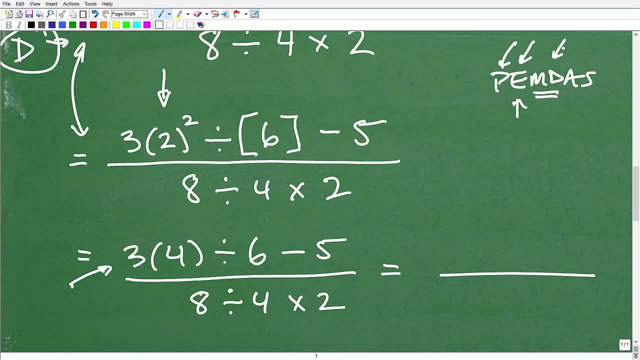 to look at multiplication and division. remember, i'm going to look at this as a bundle, right, so it's. So is there any multiplication and division? Yes, there is. This is multiplication, and then I got division here, So which comes first? Okay? 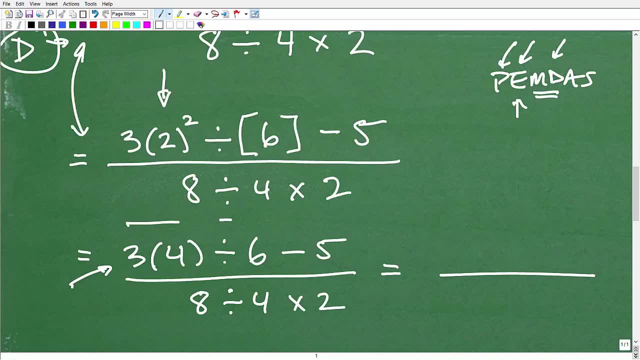 Well, multiplication comes first from left to right, So we're going to go ahead and write that down there. So 3 times 4 is 12 divided by 6 minus 5.. Then I have here 8 divided by 4 times 2.. 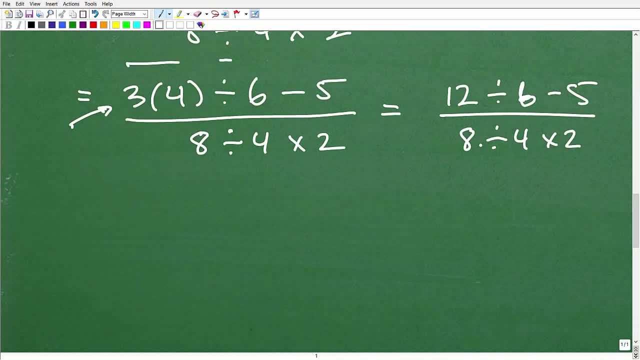 Okay. So now we're really getting there right, Getting more and more simplified, And I'm going to write this down here: 12 divided by 6 minus 5 over 8 divided by 4 times 2.. All right, 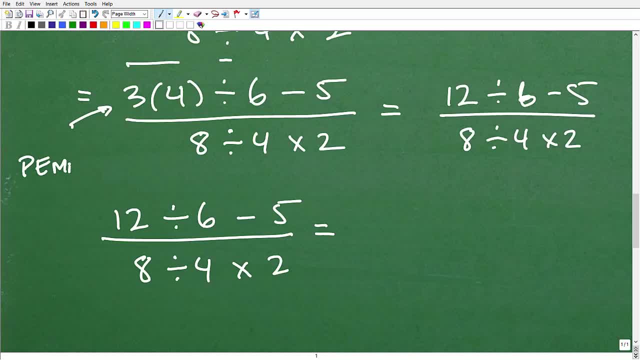 So let's get our little PEMDAS out again. P-E-M-D-A-S. So let's go back to our M and D. Just because we just did a multiplication, It doesn't mean that we're going to move on to addition and subtraction. 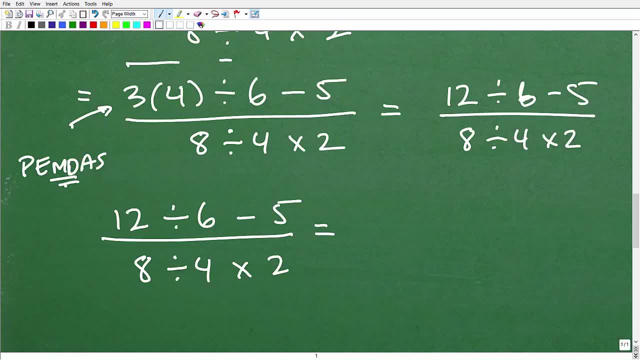 We have to exhaust all situations that involve multiplication and division. So we're looking again. I'm focused on the numerator. Is there any multiplication or division? Yes, there is division going on here, So 12 divided by 6 is going to be 2.. 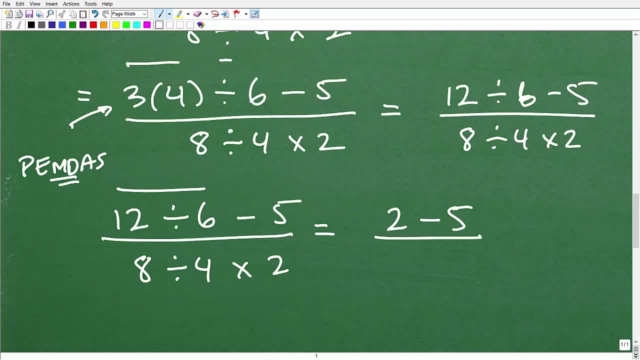 So this is going to be 2 minus 5, okay- over what's going to go on in the denominator. So this is a good opportunity to deal with the denominator right now. So let's kind of start working on that, Okay. 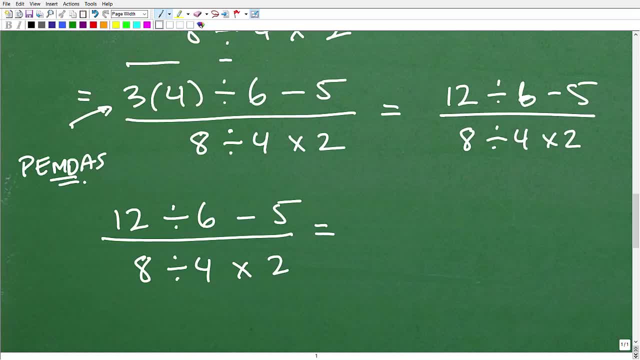 Let's go back to our M and D. Just because we just did a multiplication doesn't mean that we're going to move on to addition and subtraction. We have to exhaust all situations that involve multiplication and division. So we're looking again. I'm focused on numerous. Is there any multiplication or division? 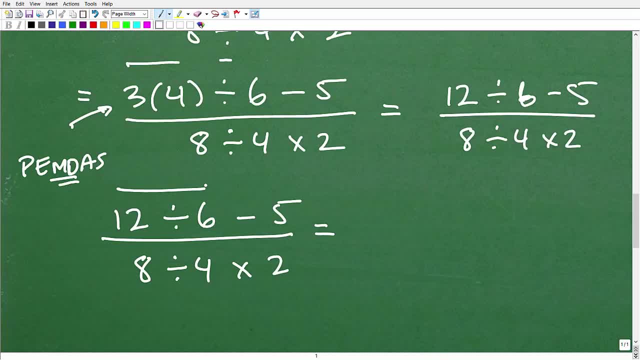 Yes, there is division going on here. So twelve divided by six is going to be two, So this is going to be two minus five, OK, Over what's going to go on in the denominator. So this is a good opportunity To deal with the denominator right now, So let's kind of start working on that. 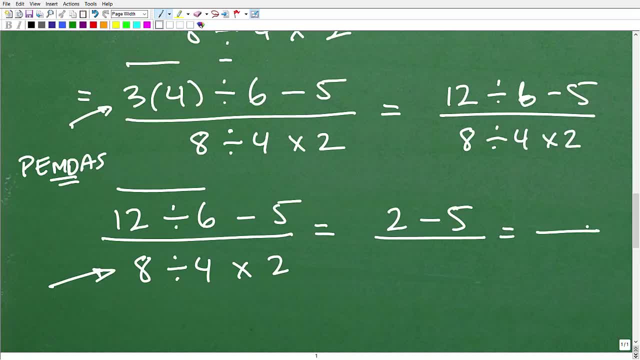 OK, so two minus five. We know our final answer here is going to be what. What is two minus five? A little pop quiz for you. So if you said three, you would be perfectly incorrect. OK, it's not three, It is negative three. 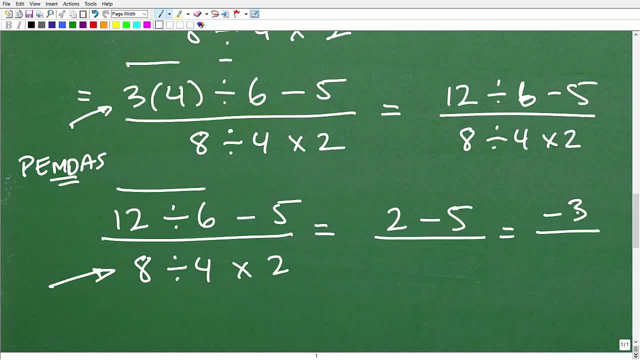 So watch your positive and negative number rules. OK, and that's what I'm talking about. If you made that error, then you've got to slow down and just keep focused On all the little details of this problem. So let's focus in on the denominator. 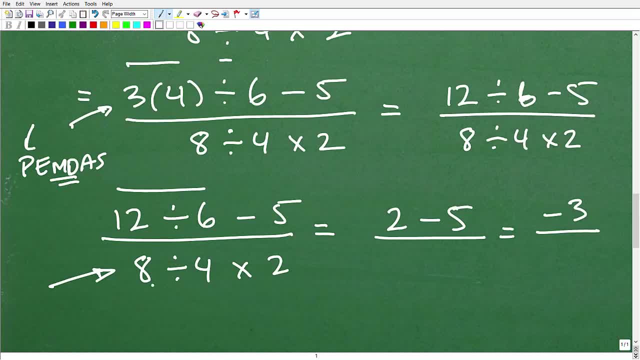 So I have. Do I have any parentheses? No, I do not have any parentheses. Do I have any exponents? Nope, no exponents. Do I have multiplication division? Yes, that's what I have: Division and multiplication. So this time I have division before multiplication. 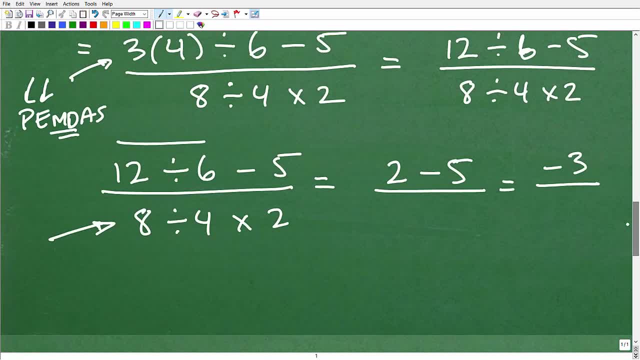 See, a lot of students would make this error. Let's just do this wrong here. for a second, What if we did the multiplication first? We would get eight divided by eight, which is going to be one, right? So if I did multiplication and then division, OK it would be, the denominator value would be one. 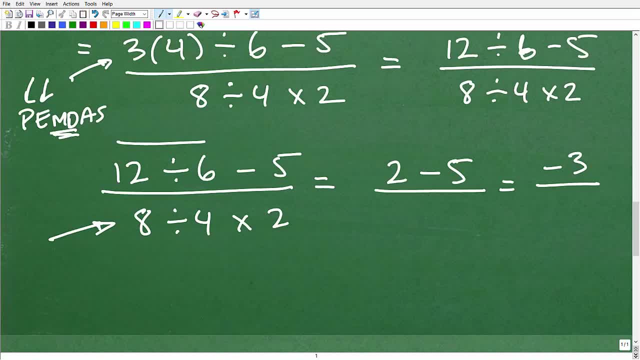 But that's not what I'm supposed to do. OK, I'm supposed to do whatever comes first from left to right. So division comes first. So I have to do eight divided by four. So that's going to be two, OK, and then I have this multiplication. 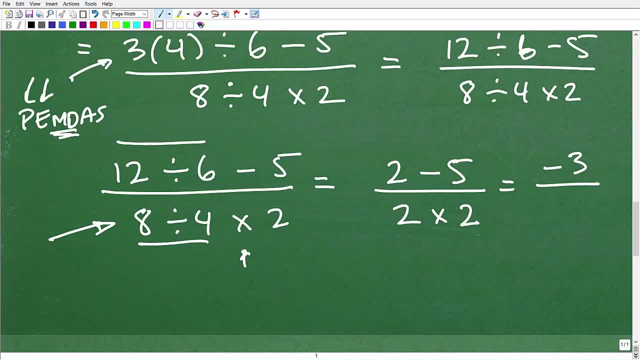 So two times two, All right. So two times Two is obviously going to be four. This is my final answer. But you can see if I would have went the other route. if I did multiplication first, I would have had eight divided by eight, or one. 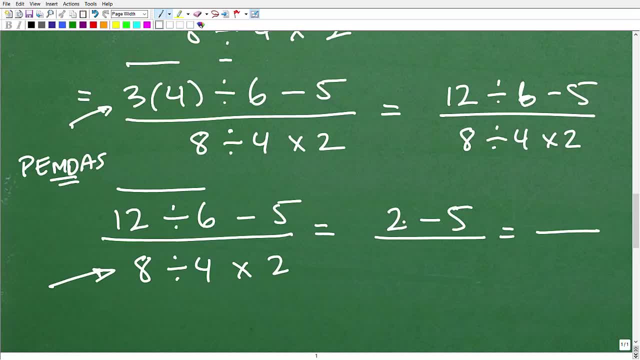 So 2 minus 5, we know our final answer here is going to be what. What is 2 minus 5?? A little pop quiz for you. So if you said 3, you would be perfectly incorrect. okay, It's not 3.. 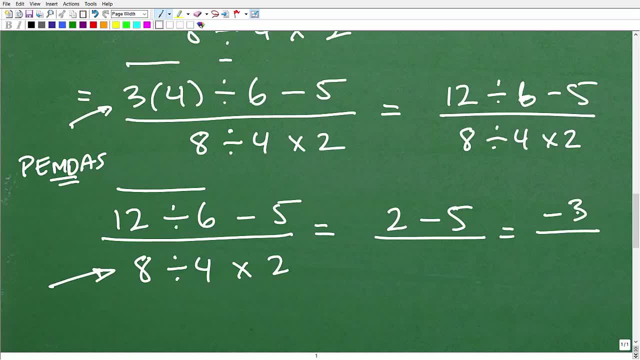 It is negative, 3. So watch your positive and negative number rules. okay, And that's what I'm talking about. If you made that error, then you've got to slow down and just keep focused on all the little details of this problem. 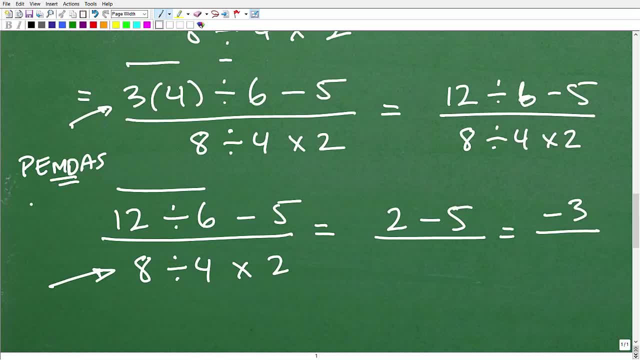 So let's focus in on the denominator. So I have. do I have any parentheses? Nope, I do not have any parentheses. Do I have any exponents? Nope, No exponents. Do I have multiplication and division? Yes, That's what I have. 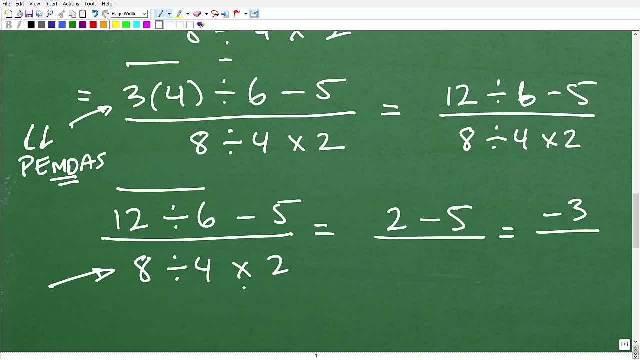 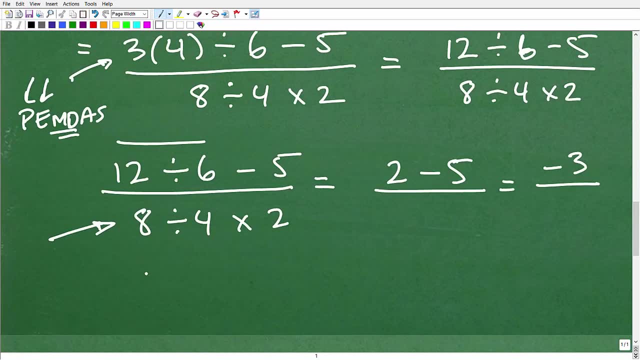 Division and multiplication. So this time I have division before multiplication. See, a lot of students would make this error. Let's just do this wrong here for a second. What if we did the multiplication first? We would get 8 divided by 8, which is going to be 1, right. 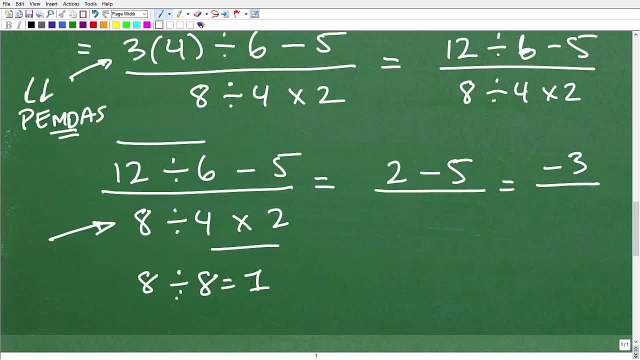 So if I did multiplication first, what would I get? 8 divided by 8, which is going to be 1, right? So if I did multiplication and then division, okay, it would be. the denominator value would be 1.. 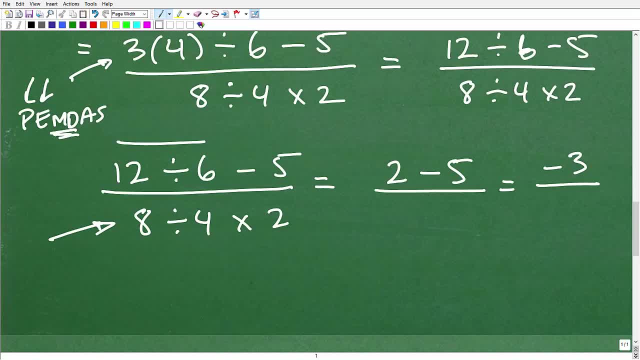 But that's not what I'm supposed to do, okay, I'm supposed to do whatever comes first from left to right. So division comes first. so I have to do 8 divided by 4.. So that's going to be 2, okay. 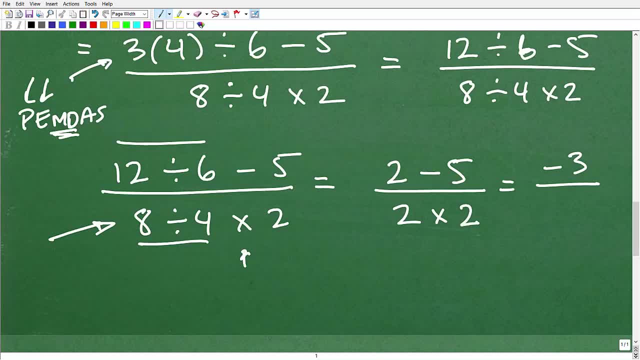 And then I have this multiplication. so 2 times 2, all right. So 2 times 2 is obviously going to be 4.. This is my final answer, but you can see if I would have went the other route. If I did multiplication first, I would have had 8 divided by 8, or 1, okay. 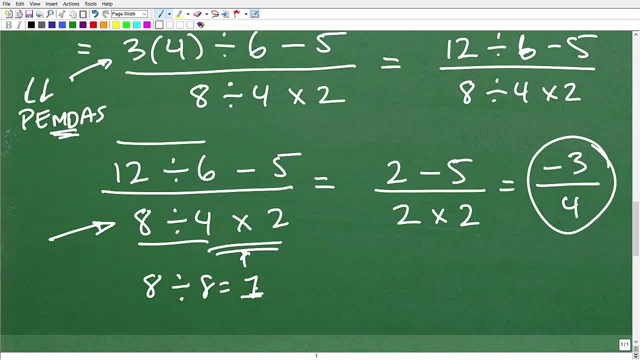 You would have gotten the wrong answer. There is a very specific- you know- order that we have to take when we're dealing with all these mathematical operators. That's why we have the order of operations and, thank goodness, our Aunt Sally is helping. 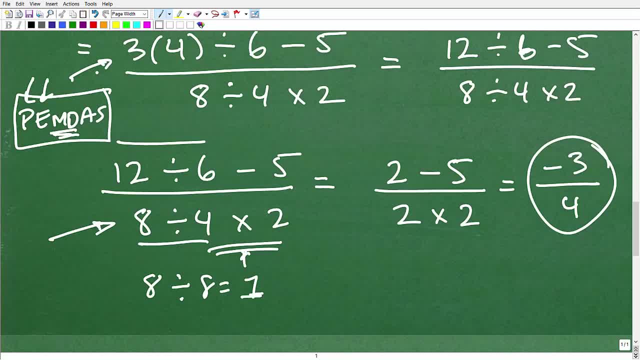 us out here, right? So please excuse my dear Aunt Sally, but I think Aunt Sally sometimes didn't fully explain how she wants us to use This recipe book. you know like hey, again, you know some of the biggest misunderstandings. 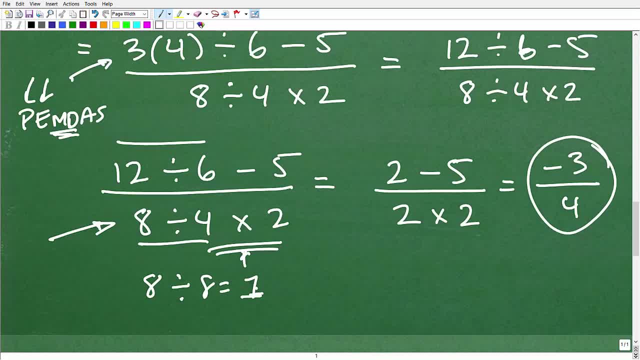 OK, you would have gotten the wrong answer. There is a very specific- you know- order that we have to take when we're dealing with all these mathematical operators. That's why we have the order of operations And thank goodness our Aunt Sally is helping us out here. 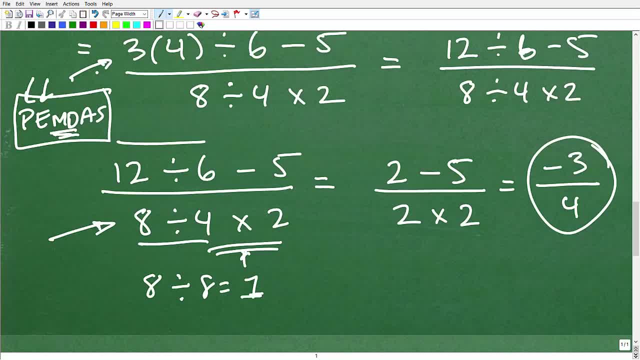 Right. So please excuse my dear Aunt Sally, But I think Aunt Sally sometimes didn't fully explain how she wants us to use this recipe book. You know like hey, again. you know, some of the biggest misunderstandings I think is with the grouping of multiplication and division and addition and subtraction. 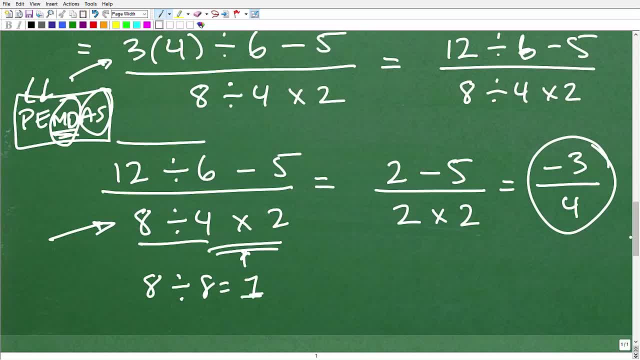 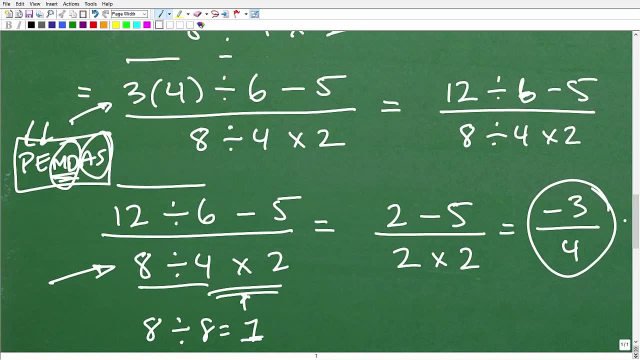 Again: left to right, left to right, All right. So hopefully you've kind of picked up. That's why I wanted you to do this problem first, because I wanted to see if you were going to make Any errors, maybe any of these errors, if you made those errors. 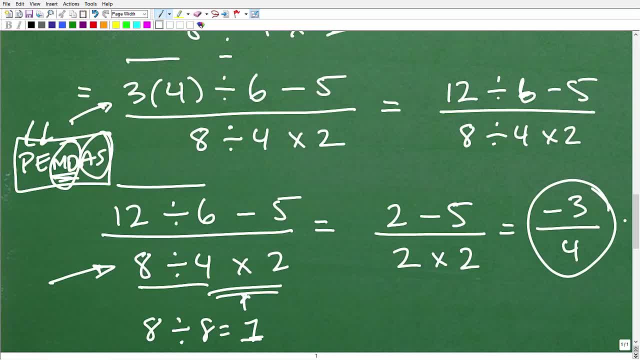 OK, I'm glad you made those errors while watching this video, because you know you should learn from them. OK, just because you made a mistake, it's not the end of the world. OK, what's critical is: are you learning? 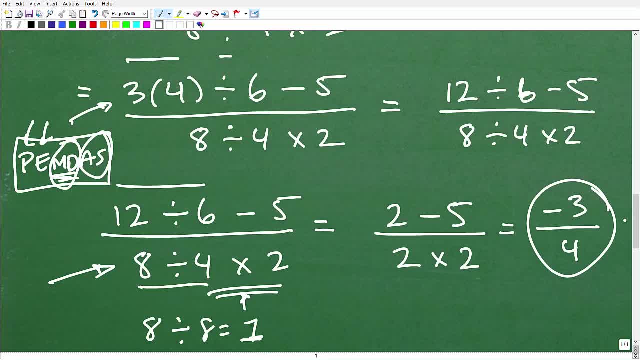 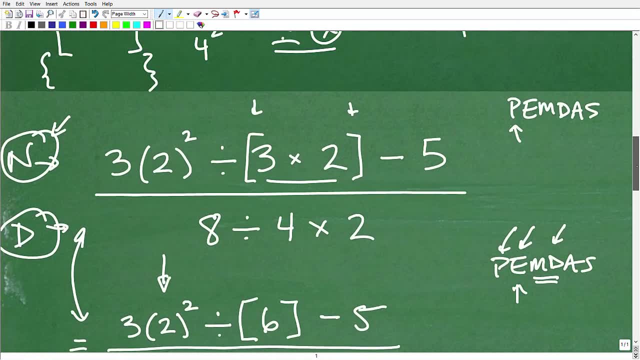 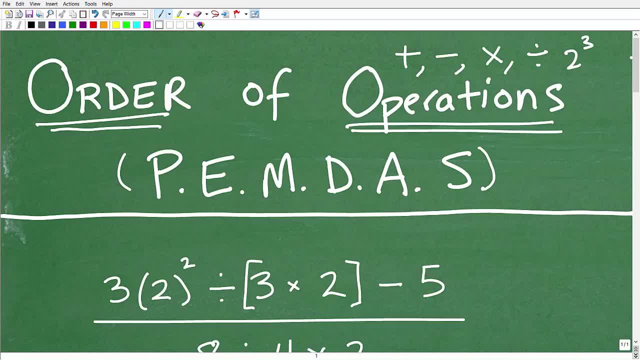 I could tell you right now this is definitely the top. if I had to say, pick the top five areas where all math students make mistakes, I would say: order of operations is, you know, right up there on one of the top ones. OK, so anyways, hopefully this little review, you know, you know, got you on the right path in terms of operations, just because we're just working with numbers and not variables or anything else like that. 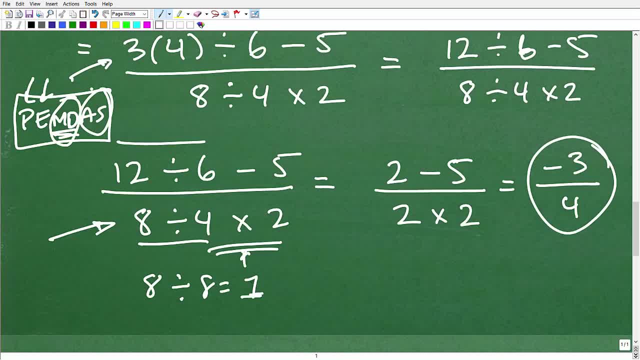 I think is with the grouping of multiplication and division, addition and subtraction, again left to right, left to right, All right. so hopefully you've kind of picked up. That's why I wanted you to do this problem first, because I wanted to see if you were. 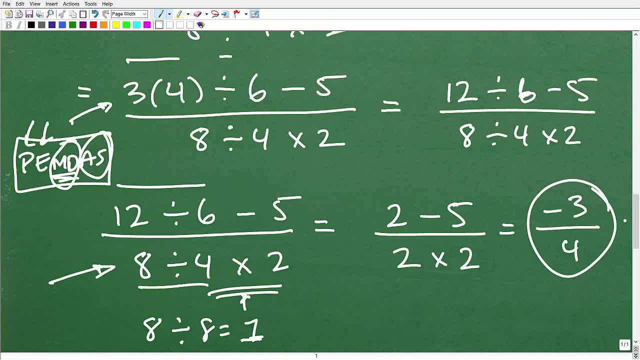 going to make any errors, maybe any of these errors. If you made those errors, okay, I'm glad you made those errors while watching this video, because you know you should learn from them. okay, Just because you made a mistake, it's not the end of the world, okay. 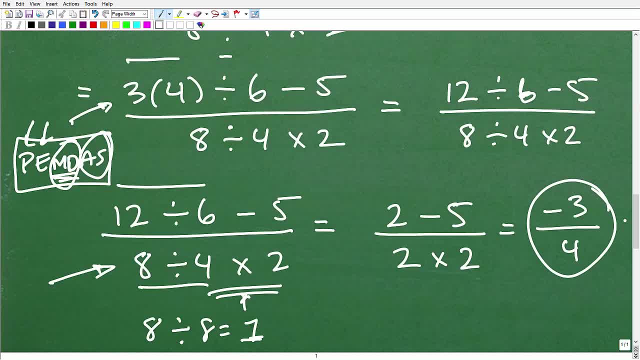 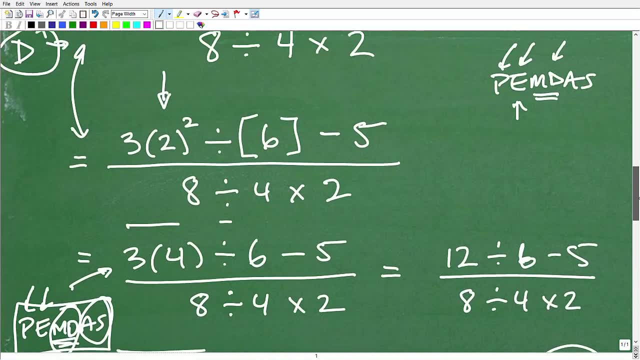 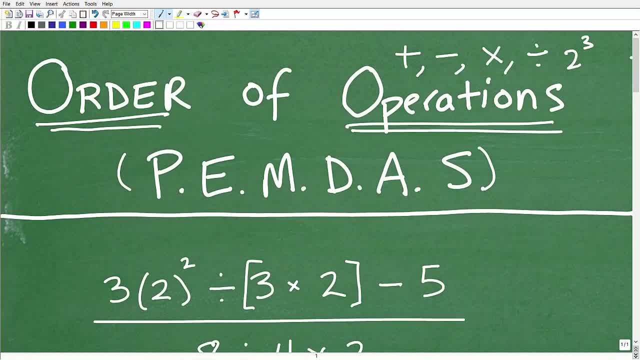 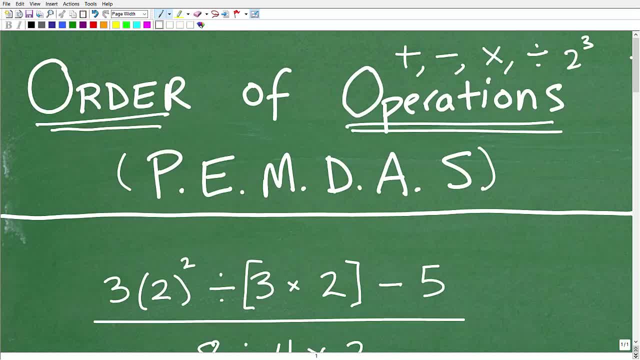 The top five areas where all math students make mistakes. I would say. order of operations is, you know, right up there one of the top ones. okay, So anyways, hopefully this little review, you know, got you on the right path in terms. 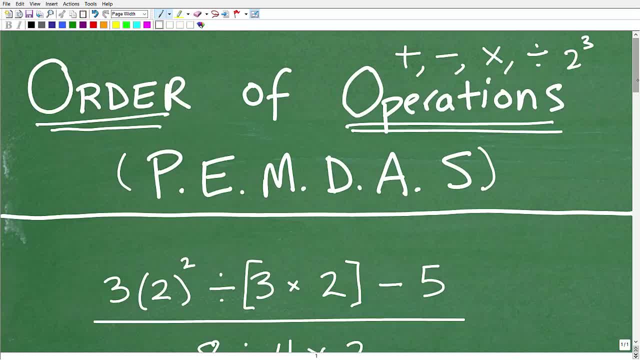 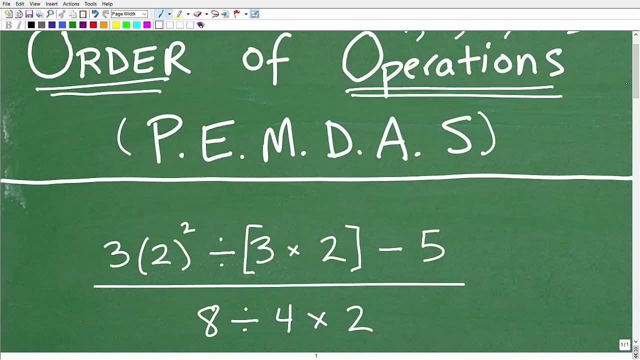 of order of operations Just because we're just working with numbers and not variables or anything else like that. don't minimize, you know, the focus and effort you know and concentration level you have to have. okay with order of operations. 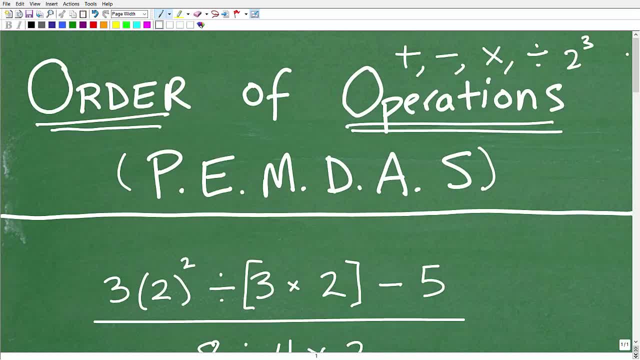 Again, show your work no more than say two steps at a time. okay, Right now, when you're starting to learn this, just one step, nice and neat. double check, just work the problem. kind of whittle it all the way down until you have your final. 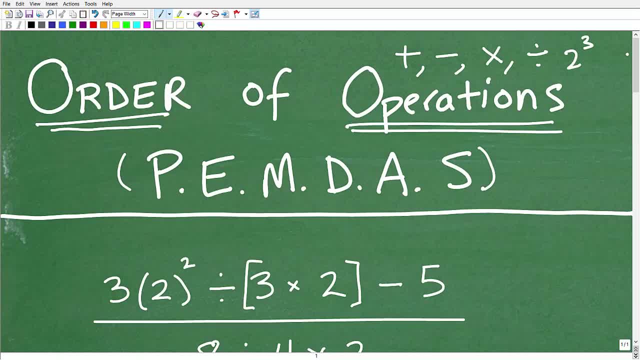 answer okay. All right, so hopefully this video helped you out. I wish you all the best in your mathematical adventures. Thank you for your time and have a great day. 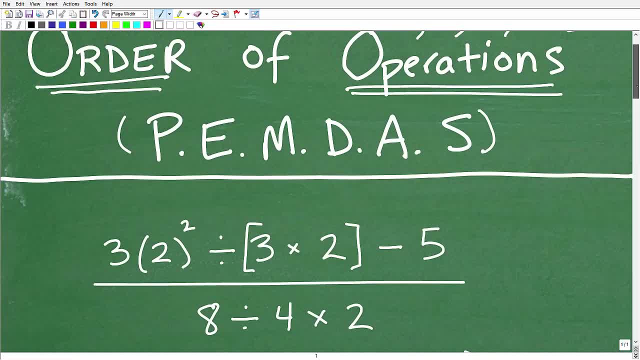 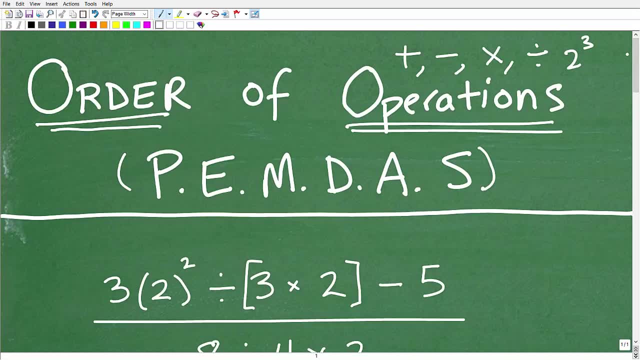 Don't know. Now minimize, you know, the focus and effort you know and concentration level you have to have. OK with order of operations. again, show your work no more than say two steps at a time. OK, right now, when you're starting to learn this, just one step.